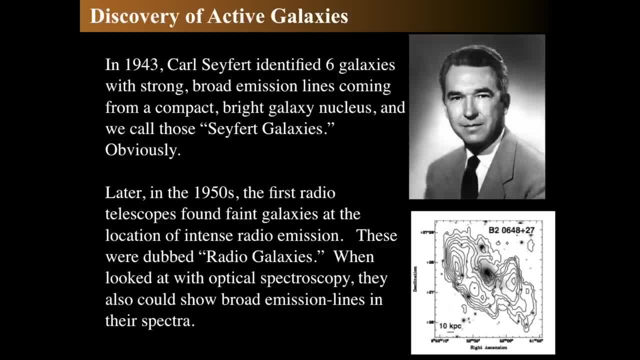 He studied galaxies that had strong, broad emission lines and they came from the center of the galaxy, meaning mostly, coming mostly from the center, meaning the nucleus of the galaxy, and they were bright and compact galaxies. Those are called Seifert galaxies because, you know, 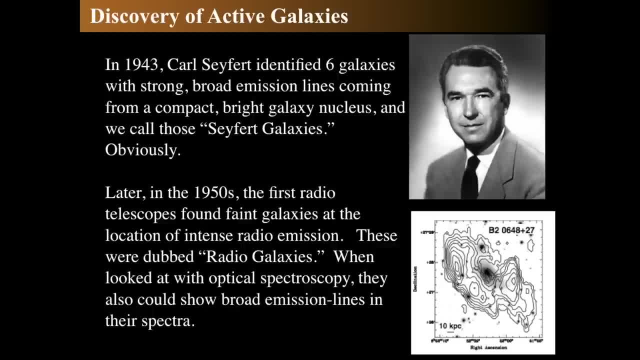 the guy who discovered them were Seifert. Well, in the 50s radio telescopes found that some of the faint galaxies that were there were many, many, many faint galaxies found at the location of extraordinary radio emission And they're called radio galaxies. 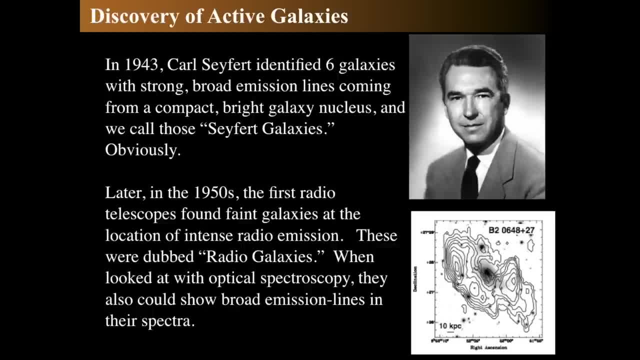 Okay, so kind of had names. We had names for things before we really knew what they were. But so there were Seifert galaxies with broad emission lines and radio galaxies doing a lot of extra radio emission. But the thing is is that when you look at with optical spectroscopy 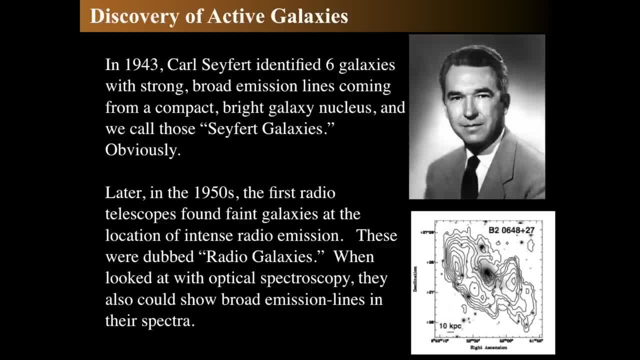 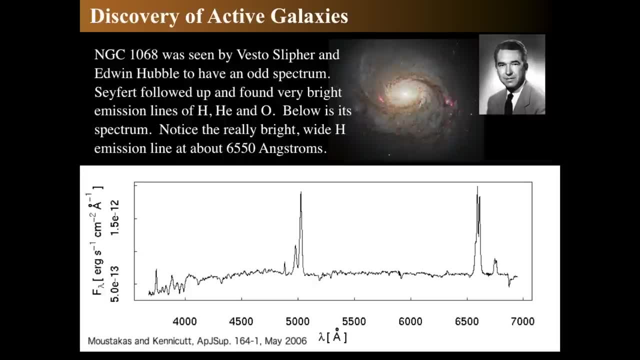 we see that there's broad emission lines in their spectrum. So what he did back in, actually, why did Carl Seifert actually go and look at these things? Well, back in the day, prior to the 1920s and 1930s, 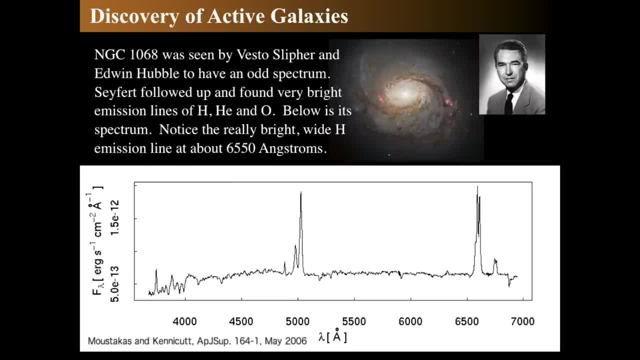 Vesto Seifert and Edwin Hubble looked at a specific one, one of the nearby galaxies, NGC 1068, which is one of the Messier objects- I believe it's Messier 77,- found it to have a really weird spectrum. 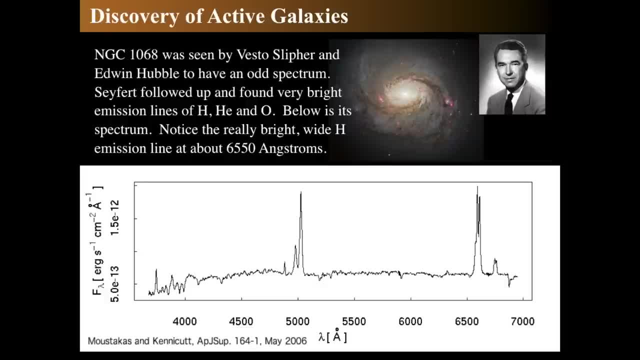 And that's an odd thing. And what they did is that Seifert did do the follow up And this was one of his first galaxies that he looked at And he found that it had big emission lines of hydrogen, helium and oxygen. 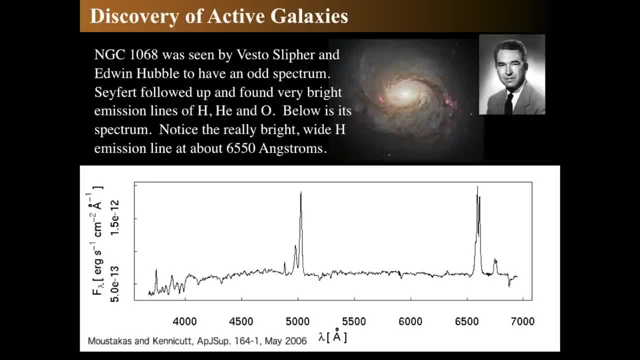 And this is a more modern version of its spectrum taken by Mostakis and Connecticut back in 2006.. And we find, if you look closely, that there are some really, really bright hydrogen emission lines, specifically the one at 6,550 angstroms. 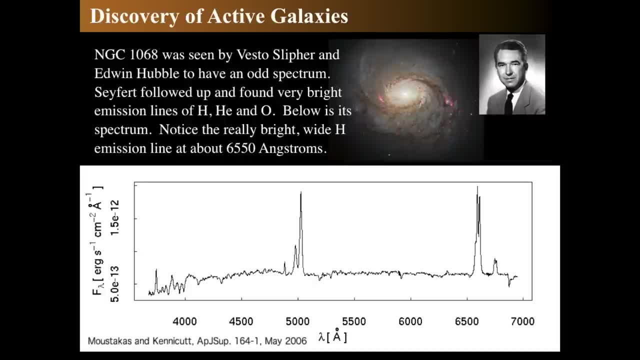 That is hydrogen. We also see the helium line at 5,000, and there's also some other bright oxygen lines floating around in there too. But notice, it just kind of has a flat spectrum from left to right, unlike the star spectra that we saw. 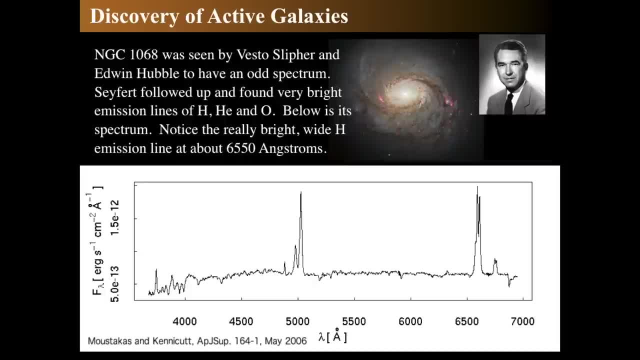 So this is a very different sort of spectrum And notice, the hydrogen emission is extraordinarily wide. That wouldn't look pink, That would look kind of reddish, but it wouldn't have that distinct pink that we associate with those star-forming regions like we see in the spiral arms of this particular galaxy. 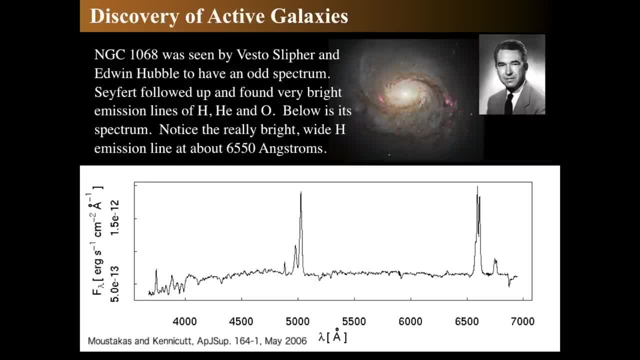 So look at that little inset image and you see that there's these pink glows. Those are star-forming regions and that's the pink stuff. Now, that is also at the wavelength of 6,563, but notice the intensity of the light at that one specific wavelength. 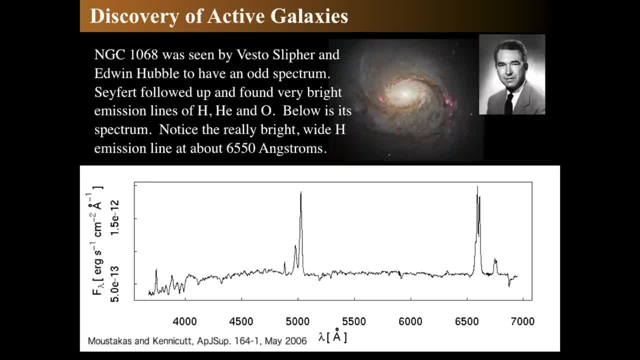 Also then compare, Compare it with the bright kind of yellowish-whitish center of the nucleus. The nucleus that we see in the inset is the place where this spectrum comes from. If we were to look at just the pink clouds off to the right hand of the center, we would only see a bright pink thing. 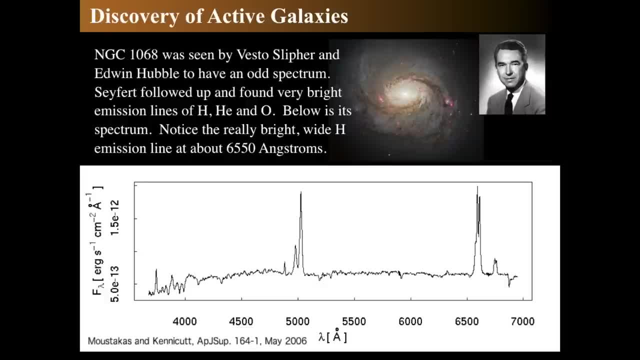 So at that specific wavelength we wouldn't see much else. That's why it looks that pinkish color. But the bright center of the galaxy has enormous hydrogen emission, which is very broad, as well as emission at other wavelengths too. But that's right down in the center. 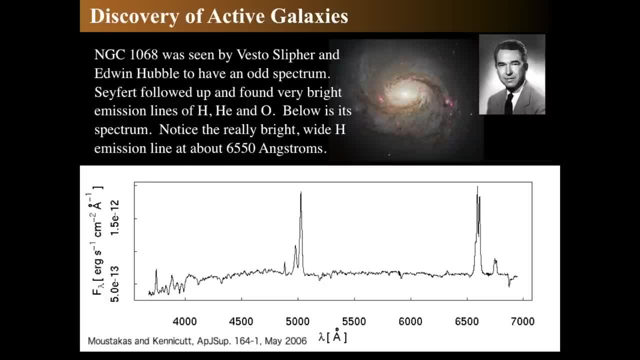 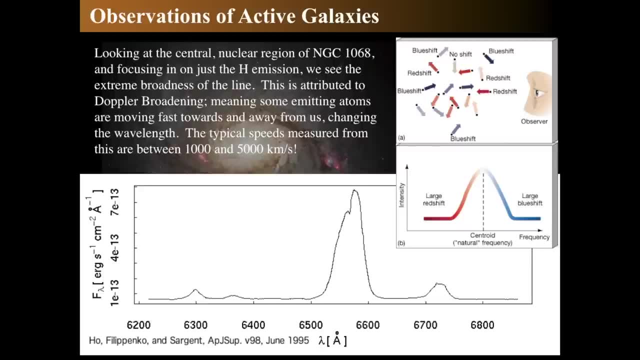 So it doesn't look pink though, which is really interesting. That's because it's bright at many wavelengths. All right, So if we then zoom in and look at just that central region, just that tiny, tiny dot in the center, 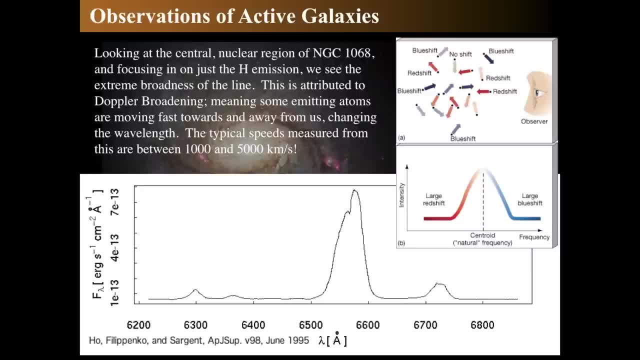 not the outskirts but the really bright center of the image of that galaxy. we find and focus in specifically on the wavelength band only for hydrogen emission. You can then see just how broad the image is. You can then see just how broad the image is. 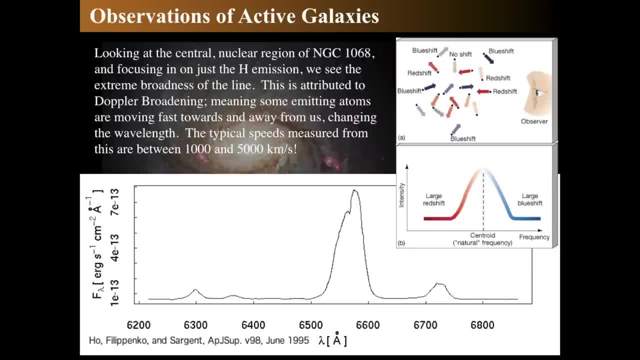 You can then see just how broad the image is, And that's what the emission line is. It's not just at six, five, six, three angstroms, It's really smeared out and much, much wider. So it's almost 100 angstroms wide and more like 50 or 60 angstroms wide. 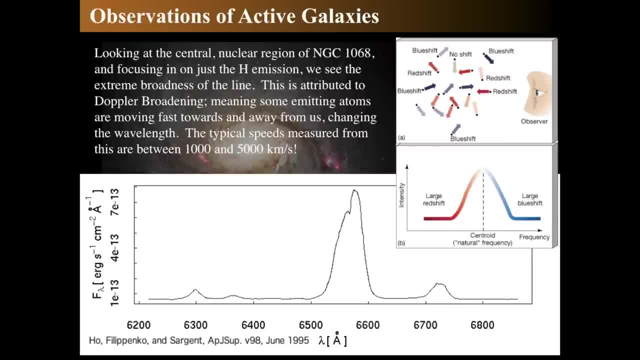 When an emission nebula like the Orion Nebula or something like that, will only be about five or ten angstroms wide. So this broadening is due to what we call Doppler broadening, And Doppler broadening means that there's some clouds of gas that are moving towards us. 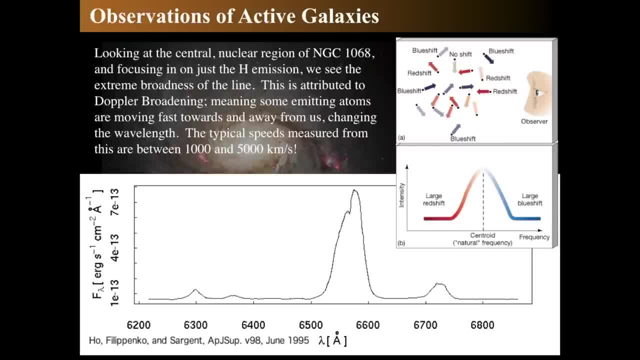 and some clouds of gas that are moving away from us. them are moving extraordinarily fast, up to 5,000 kilometers per second. So how does that make it broad? Well, as you can see, in the inset we've got some cloud. now we can break it down to individual. 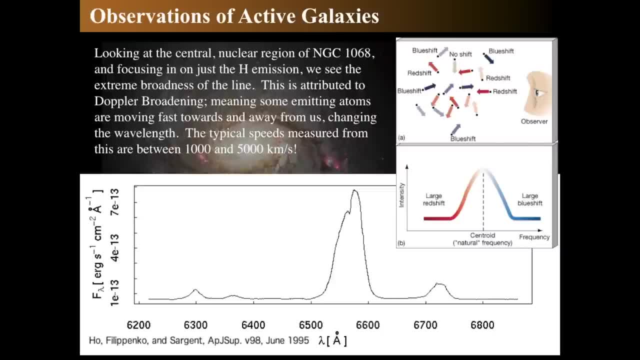 particles inside the cloud and we see that if well, bulk clouds. but let's just pretend we're looking at each of these dots as one individual cloud. So if it's really moving fast, then the hydrogen, and if it's moving fast towards us, the hydrogen. 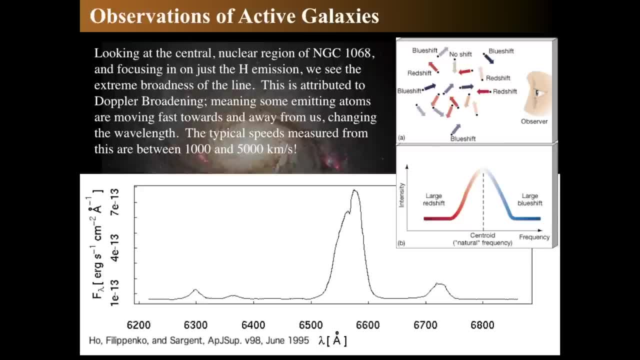 can absorb light, that would or emit light. this is all an emission now the emission from a hydrogen atom moving very quickly towards us. its wavelength of light will be blueshifted and hydrogen moving very quickly away from us will be strongly redshifted. 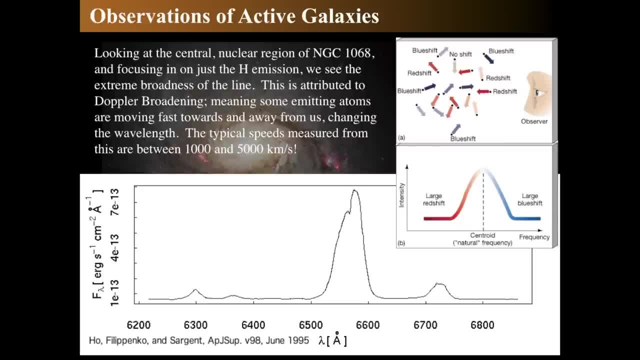 Now it's a mix between high redshift and low redshift, but mostly in between. so that's what the color combination is trying to show in the image. So the average is going to be blue. The average is going to be kind of right on the center of it, because the average is definitely 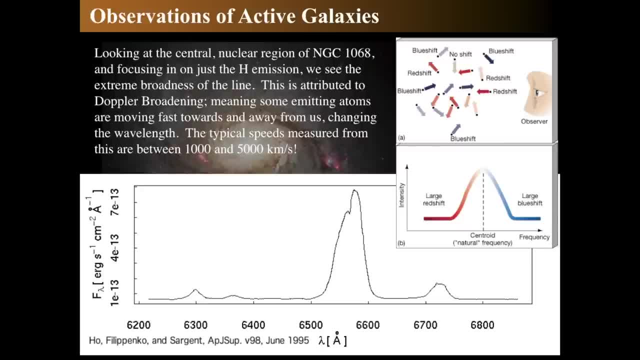 on the center, but there's some high moving parts and some low moving parts. However, when we're looking at the central region of this galaxy, it's not really that it's whole huge clouds such as the pink dots, but they're really really, really tight in. 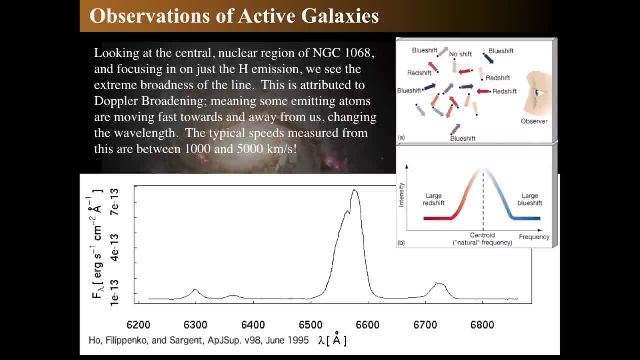 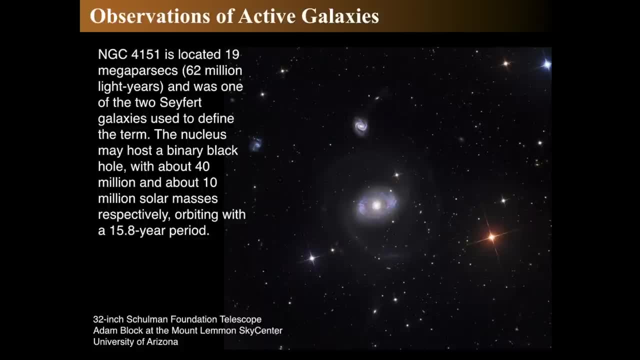 and they're really compact, and so they're moving extraordinarily fast and they're extraordinarily bright. All right, so let's see some other observations of some other Seifert-type galaxies which are really pretty. So in the center of this image We see NGC 4151,, which is about 62 million light years away. 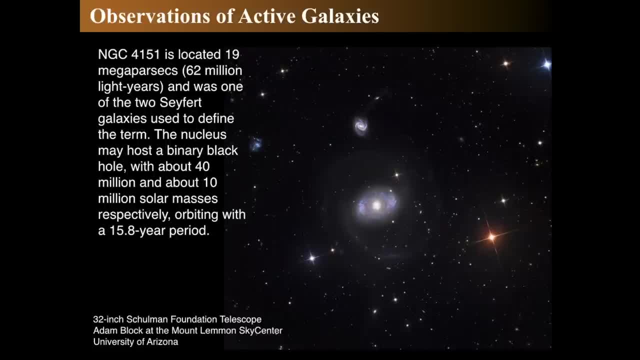 This picture was taken by Adam Block with the Mount Lemmon Sky Center at University of Arizona, and it was taken on a 32-inch scope of the Shulman Foundation Telescope. Now we- in fact this was another one of the core group that Seifert additionally used- 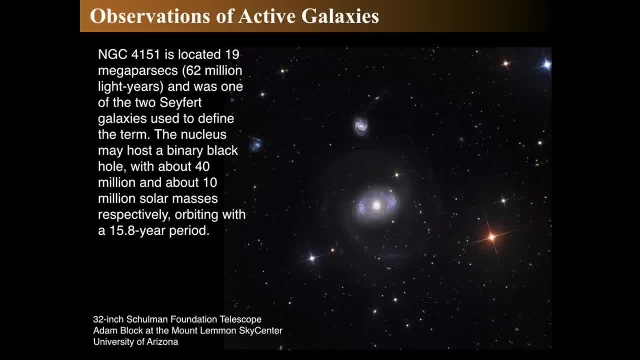 to define the term a Seifert galaxy. Now we are going to say this a couple of times, that the nucleus might hold a black hole. I mean, I'll allude to that in the next lecture, but let's actually step away from that step. 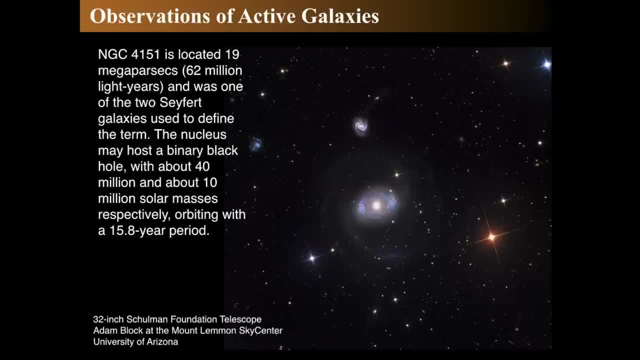 back from that idea and actually just look at the nature of what we're actually seeing. So that's actually funny is that there might be binaries that do orbit really fast. but the most important thing in this is that we've got a very, very, very bright, compact region. 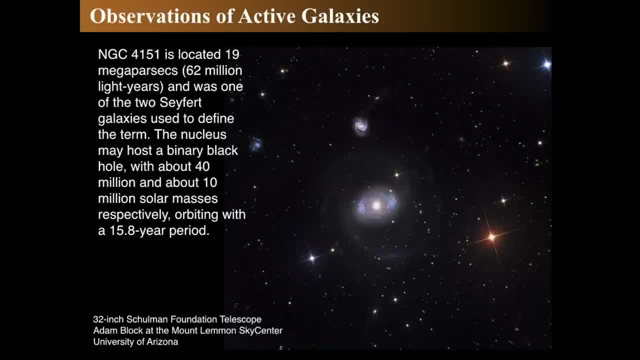 of the galaxy that has very strong emission lines and looks kind of whitish, but it's bright overall. In fact, if you look really closely at this thing, you'd guess that the center of that region is easily just as bright as all the rest of the galaxy combined. and you'd be right. 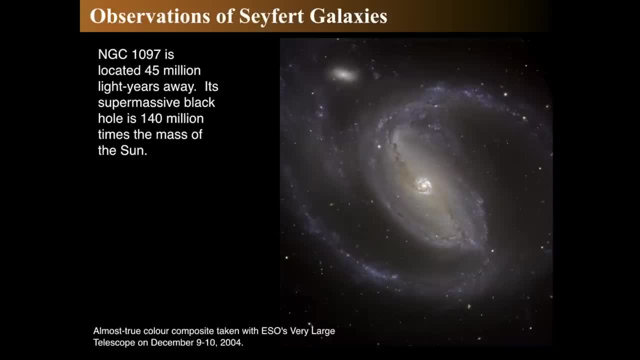 All right. another wonderful Seaford galaxy is NGC 1097.. It's an extraordinarily bright nucleus and a bar-like structure. It's about 45 million light-years away. It exhibits some of this and this picture was taken by the European Southern Observatory's VLT on a couple of nights. 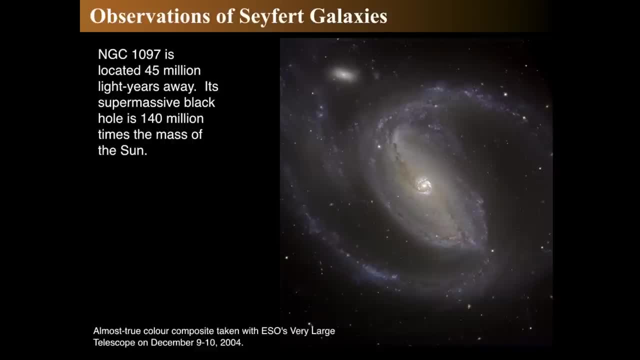 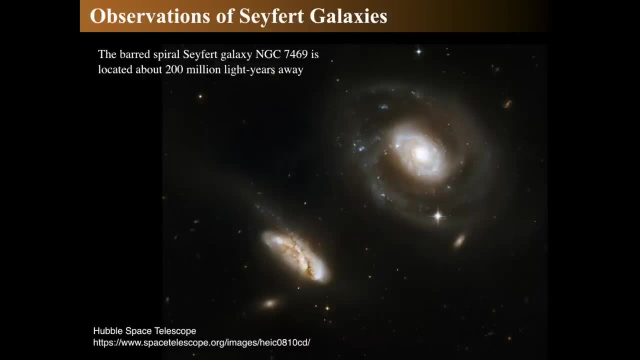 It just so happened that I believe the president of Spain was there during this observation down in Chile. This is another Seaford galaxy, NGC 7469.. It's the one on the upper right. It's actually colliding with the one that's in the lower left. This is almost 200 million light-years. 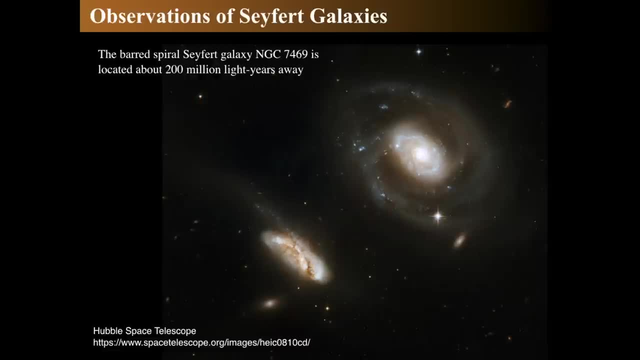 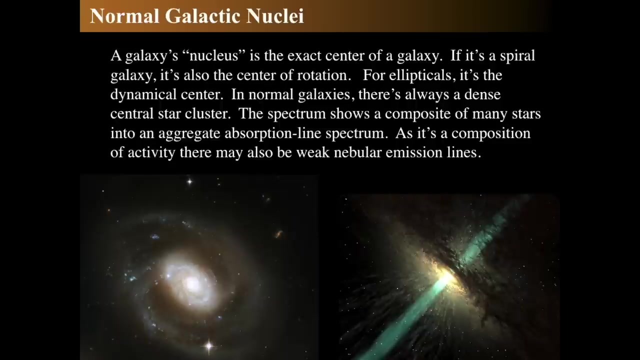 away. That's why it looks fuzzier than all the rest. It's farther away so it's harder to get it clear, And this is a Hubble Space Telescope image and that you can go check out that image with. But again we see a very, very, very bright, compact nucleus. So let's compare and 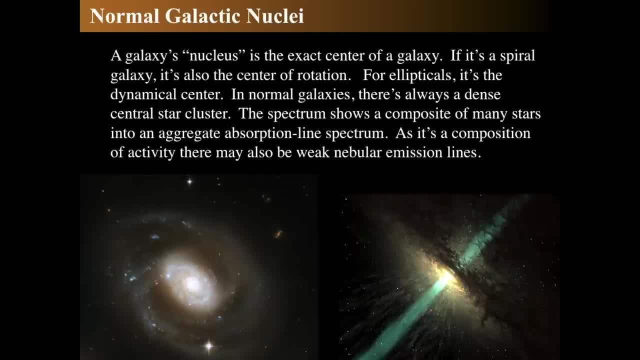 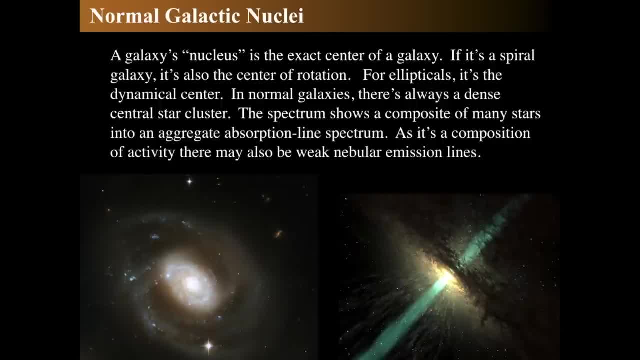 then it's the exact center of rotation of the entire galaxy. In ellipticals it's like this dynamical center around which everything seems to be orbiting, And then for normal galaxies there's always some sort of really dense star cluster in the center. Maybe there's a supermassive. 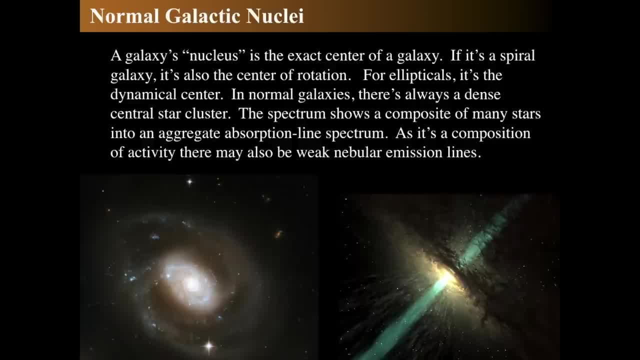 black hole, Almost always actually- And the spectrum shows of a normal galaxy: lots and lots and lots of stars and lots of absorption lines, And so there's a bunch of things happening in there. There might be gas emission and so forth, but mostly it's stars and gas and dust And it's a composition of those things, And so 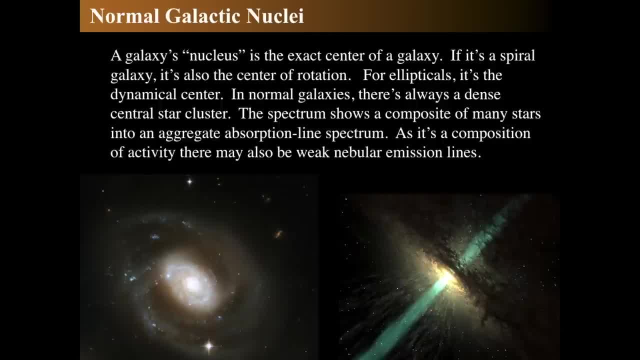 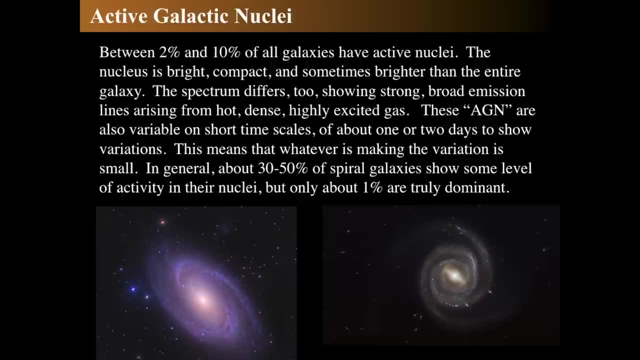 you can see that And there might be some weak nebular emission lines like the hydrogen emission lines. However, if you're looking at an active galactic nucleus, it's very different. Roughly about 10% of all galaxies have what we call our active galaxies or active nuclei. This is a really fuzzy. 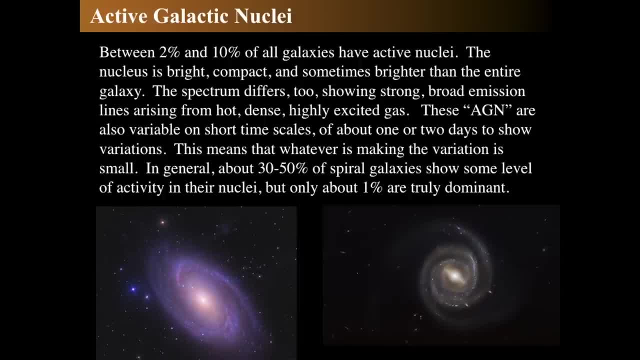 number. You look around at it and this number is very fuzzy. But the most important thing is: not all galaxies are active, But in general an active galaxy shows a bright, compact galaxy, And sometimes it's brighter than the entire rest of the galaxy. The spectrum is different too than a. 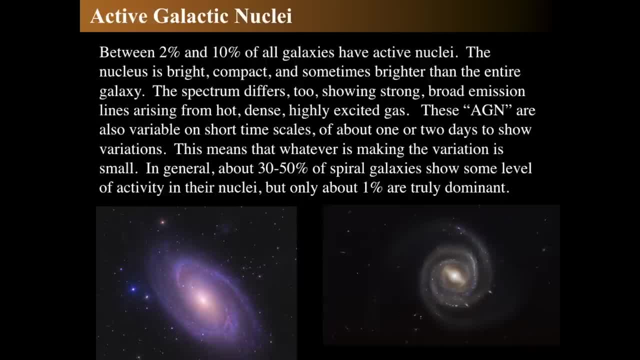 normal galaxy. There are those strong broad emission lines, like I showed you before, And they're coming from extraordinarily hot, very excited gas that's moving really fast around. So these AGN, or active galactic nuclei, they're also variable. So if you were to take a spectrum of them or their brightness, they vary on extraordinarily. 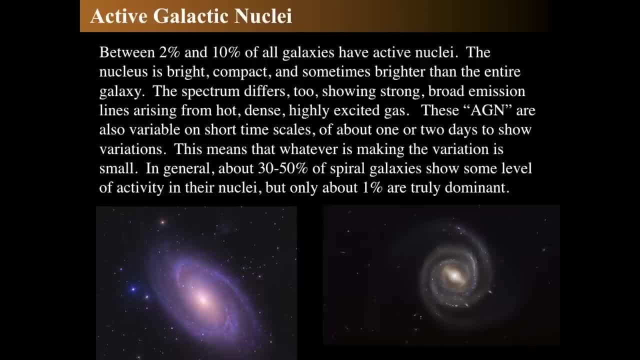 short timescales, for about a day or so. That means that whatever's making this variation is very small, meaning it has to be smaller than one or two light days across in order for it to be coherent enough that we actually see it. So spiral galaxies tend to be the ones that we see with this kind of. 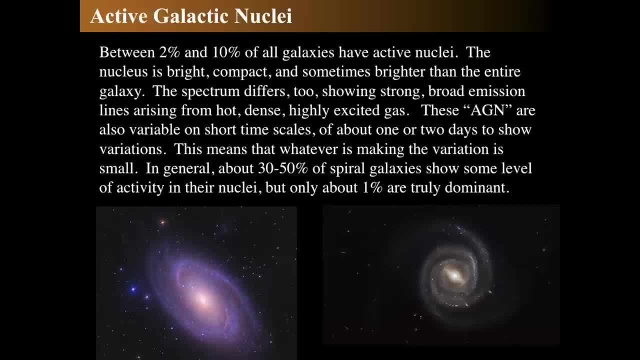 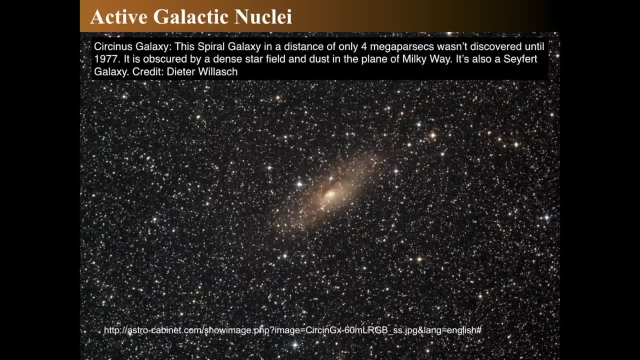 Seifert-level activity. But when we talk about really dominant cores it's only about 1% of them. So the truly dominant ones are kind of rare. An interesting one that is shown that I like to show and it's kind of one of the. 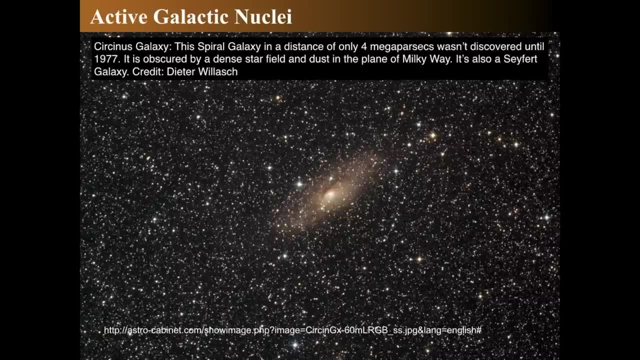 quintessential ones that you'll see in textbooks and online is the Circinus galaxy. It's a spiral that's really actually kind of close. It's only about 12 million light years away. It's one of the local, neighborhood galaxies, But it wasn't discovered because it's basically in the plane of the Milky Way until 1977. So since you're in the middle of a star field and dust plane in the Milky Way, it can easily be mistaken for some. I think in fact, you'll look in the literature and you'll find that it was mistaken for like a standard nebula. 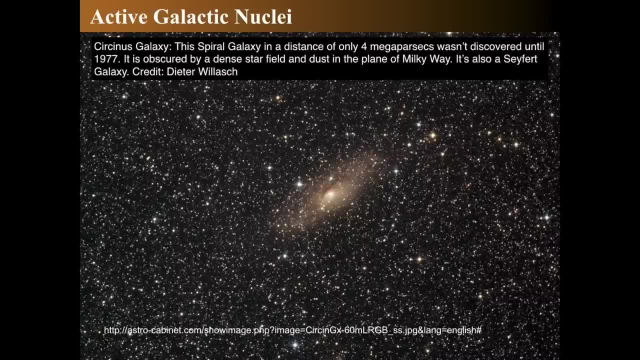 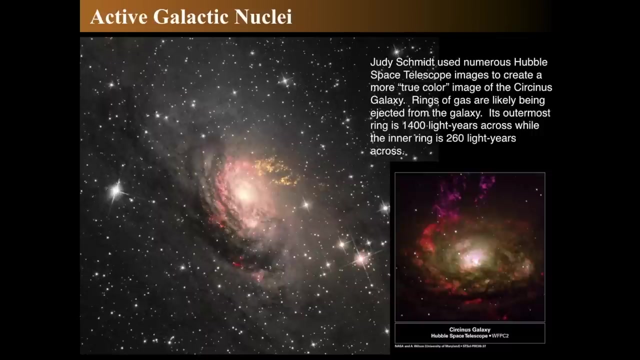 Wait a second. It's a Seifert galaxy. What do we mean by that? So let's go. in fact, let's just go back. This comes from AstroCabinet. So this is Dieter Villach. That's his work. He has some amazing, amazing stuff. I'm putting his link on the website, In any event. then there's a classic Hubble image of Seifert galaxies- the Seifert Circinus galaxy- taken with the Wide Field Planetary Camera 2. And that's what I put in the inset there, And that inset was taken with the Hubble Space Telescope by Wilson et al at the University of Maryland, And that was part of their study. So what we see, though, is that another astronomer, Judy 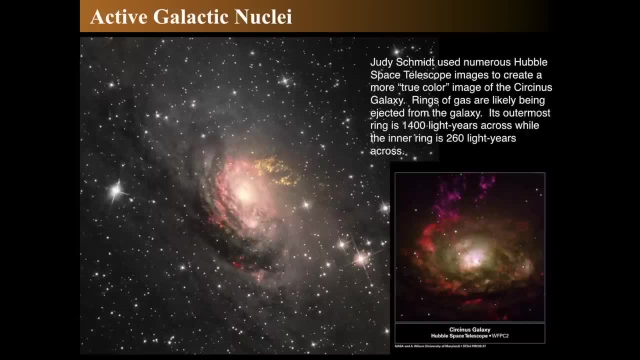 Schmidt took a bunch of the Hubble observations that were taken and then rejiggered them using Photoshop and so forth and focused in on the core and made what she considered more of a true color image. And it does look very true, colorish: The rings, and you can see the rings of the hydrogen gas And that's why it's pink, And so the rings. and then there's some ejected gas that's being shot out at high speed. in the upper right- And this is actually not a very large region- There's two kind of ringish structures. 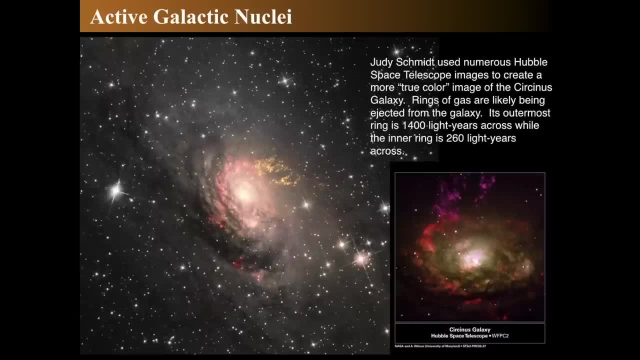 One of them is about 1400 light years across And the very deep inner ring is only about 200 light years across or 300 light years across. So really this very close by galaxy that's exhibiting extraordinary active galaxies in its active galactic nuclei is pretty close by. So we're seeing that there's some really violent things happening in this galaxy, because pretty much for the Circinus galaxy it's all about the core and it's almost nothing about the rest of it. So I invite you to go kind of hunt. 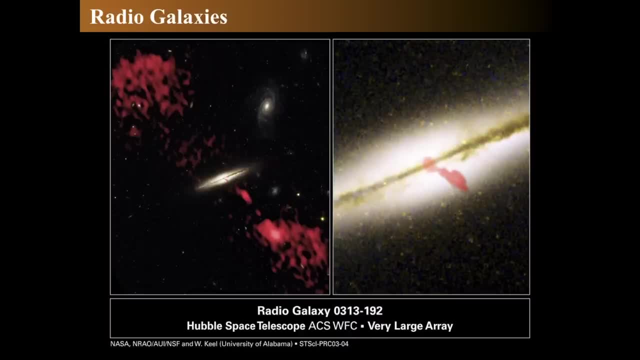 that down. I'll post the image, the link, online. So here's a and then there's another set. So Seafords were one kind of active galaxy. The other one I alluded to at the beginning were once discovered with radio telescopes. These called radio galaxies, And so we, what we see is we've got a combination of a of a NASA, NRAO and NSF image. So what we have is we have a specific, the radio emission is in red and it looks like that puffy. 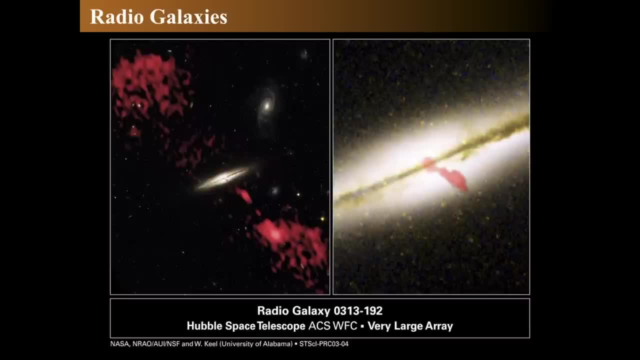 cloudy stuff. And then we have the wide field camera for the Hubble Space Telescope And that was done by Keel at the University of Alabama. But what we see is that the visual image of the wide, of the advanced camera for surveys, wide field camera, which is the, which is the kind of optical sort of view, And then we have the red puffy glow And that is the radio emission from this galaxy. So we're starting to get a hint that radio emissions very different than the rest of the emission of the galaxy. 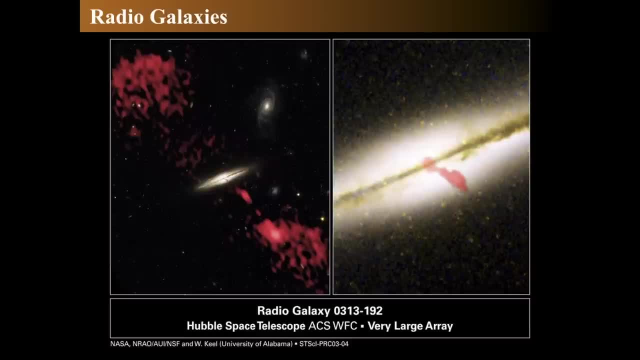 And even on the right hand side of this image we see some strong radio emission that looks like kind of a feathery sort of jutting sort of thing in the center. that seems to be bright as a dot in the center and almost like a tadpoli sort of fish thing shooting out. What's not a fish, It's a jet. So something's happening there, because those puffy clouds on either side are actually up and down or forward and back, And notice the lower right one has a little bit of a bright spot in the center. That might be where the jet which looks like a 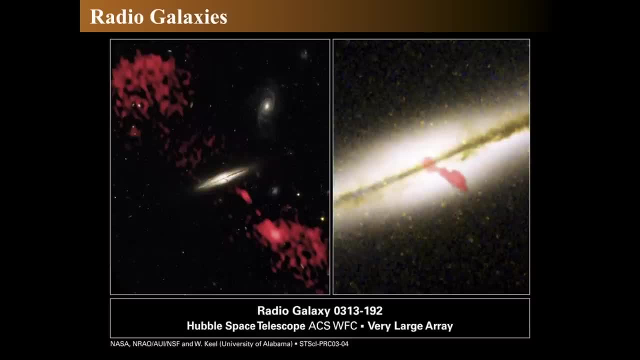 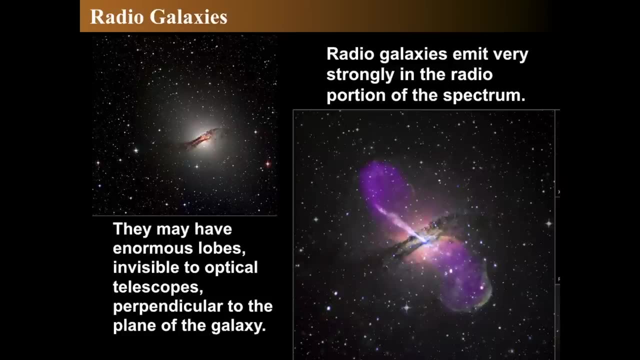 fish on the right is finally slowing down or hitting some other stuff. So let's see what we can find out about radio galaxies. Okay so radio galaxies emit strongly in the radio part of the spectrum, So that's what we think. So electromagnetic radiation, mostly in radio. So they're very strong radio emitters And they can have huge, huge, huge lobes of gas which are totally invisible optically And they go perpendicular to the plane of the galaxy, which is interesting. So you've got this. This one is called 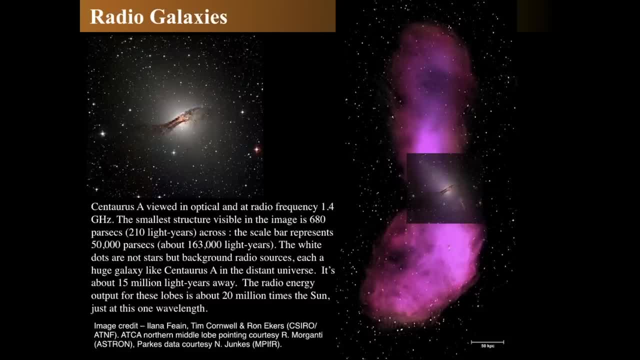 Centaurus A, And Centaurus A is one of the brightest radio sources in the sky, And on the left hand side is the image that is taken by. the upper images is a European Southern Observatory picture image, But the one on the right was taken by with the, with the Parkes Observatory as well as other observatories, to construct a very large scale image of the of the radio emission. 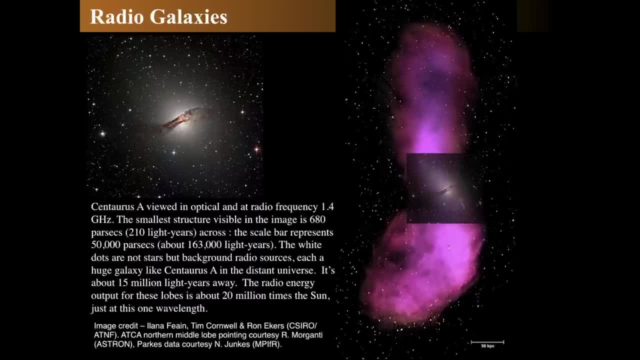 of Centaurus A. So what I did is I took the image of on the left and overlaid it with the image on the right to show you how big the radio lobes are compared to the image of Centaurus A. Now, what's fascinating is on the right is that the smallest structure, the littlest, tiniest lumps, are about 200 light years across. So it's you know these are, you know, those are big things, But yet it's pretty interesting that there is structure that's large enough to be like 200 light years across And we see a. 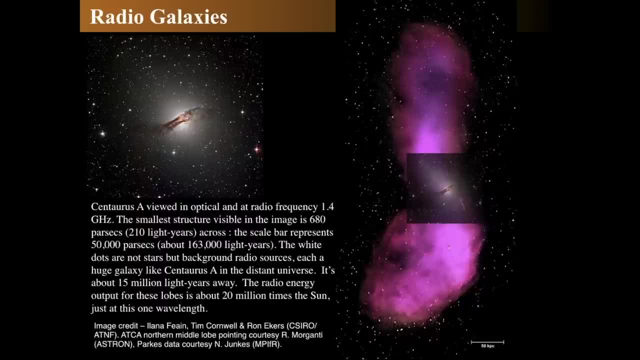 little bar at the represent that says about 160,000 light years. So that's what the bar is worth. So this thing is huge. The extent of this thing is enormous, meaning it goes over almost a million light years across, which is big. There's a lot, And because this is a radio image, the dots are not stars, Those are other active galactic nuclei, other radio sources from other massively distanced galaxies that are being 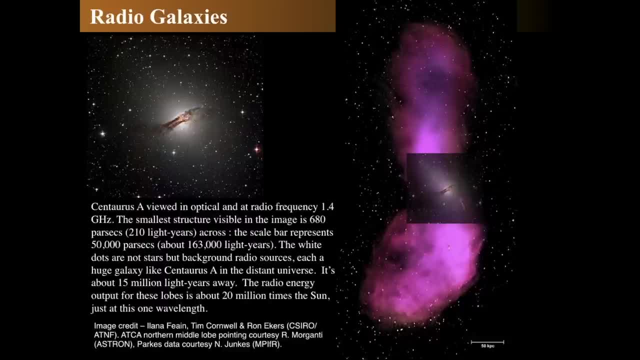 picked up by this particular telescope as it looks deep into the cosmos to make this incredible, incredible image. So Centaurus A is the pinkish glow That's the radio structure that comes from it that we do not see in visible light, And in fact, the radio energy is so incredibly large that each of the lobes is 20 million times the energy in just the radio sources as the sun puts out, And this is only happening at one time. 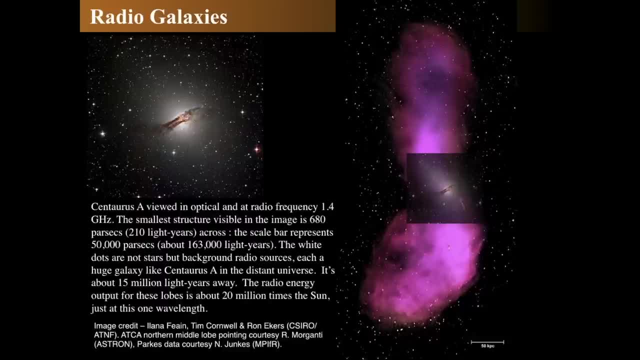 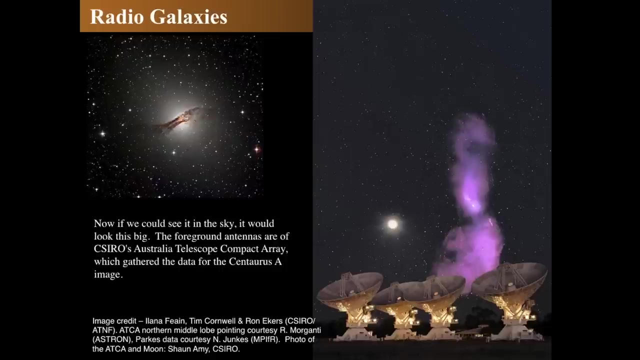 One wavelength. So 20 million times the energy of the sun's radius at, specifically, 1.4 gigahertz. So if you integrate it across all the radio emission, it's staggering amounts of energy that are being emitted. It's billions of times the mass of the luminosity of the sun If you integrate across all radio waves. All right, just for very interesting contrast, This is: this was a fascinating way they did this, And so 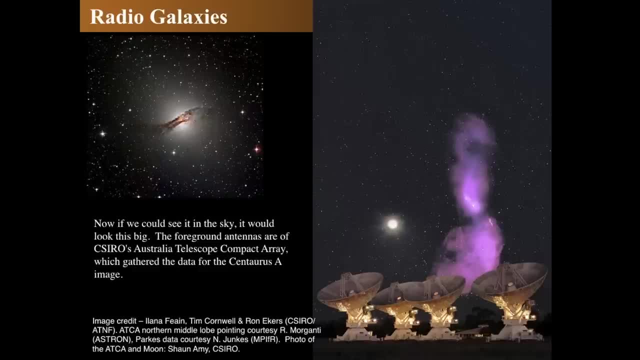 the foreground telescopes are the telescopes that were taken, that were used to take the radio image with the Australia Compact Array, And this is the image was done by Ileana Fane, Tim Cornwell, Ron Eakers, And then the northern lobe was was created with by Morganti at Astron And the Parkes Observatory data is by Junks. So the and Amy and Sean Amy at Cicero and CSIRO took the night sky image. So if you could see the Centaurus, 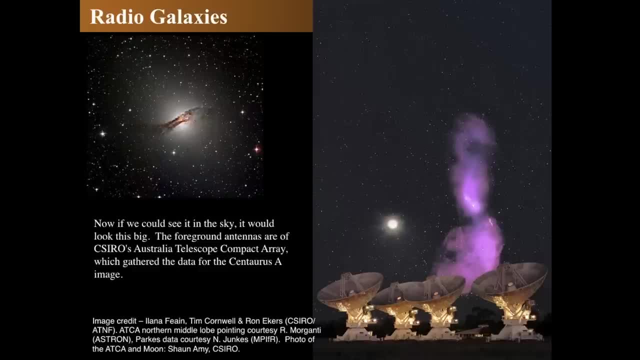 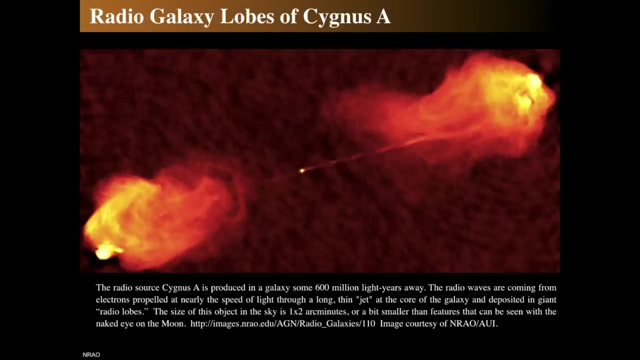 a in galaxy in the sky. That's where it would be And that's what it would look like if you could see in radio emission. The radio sky is extraordinarily different than the optical sky. It would be a vastly different place, And so, by comparison, we see the moon there in the sky. So really interesting, fascinating appearance. Other famous radio galaxies, the most, one of the most important ones, is Cygnus a. Cygnus a is a. 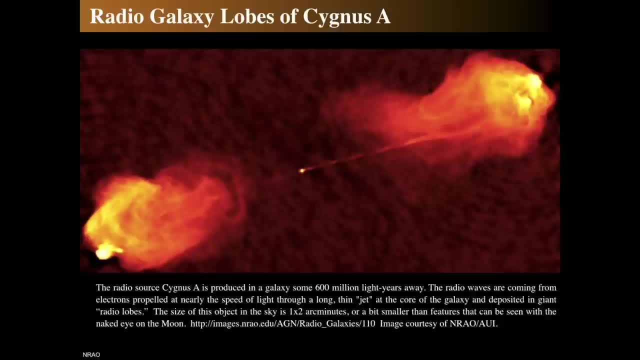 is almost, it's like half a billion light years away, and what we see is that there's a central bright core, these long jet-like structures, and then these feathery lobes at either end, and the size of this, of the object in the sky, is only one by two arc minutes. but remember an arc. 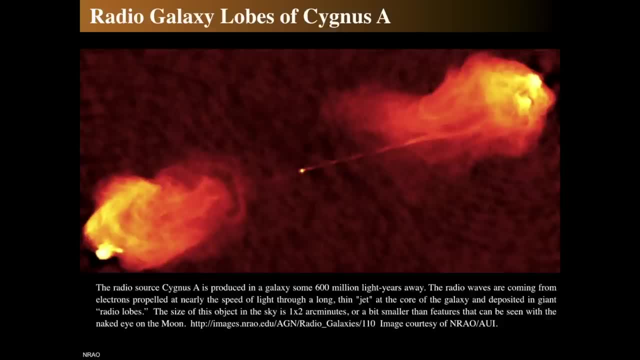 minute is the. the moon is about 30 arc minutes across, so this is only a. this would be. this image that you're looking at would be about the same size as one of the one of the smaller craters on the moon or one of the visible craters in the moon through binoculars. so if you could see radio. 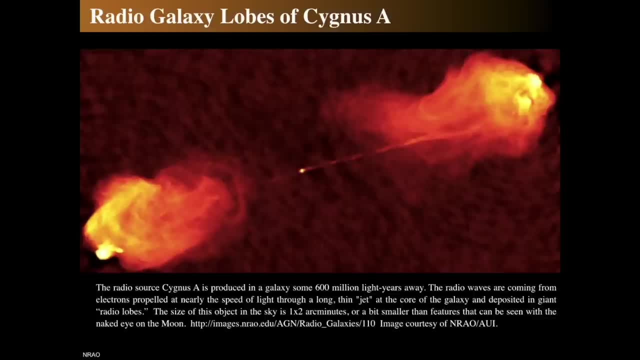 radio emission in the sky. you would see this extraordinarily bright stars in the sky. that would be that you would eventually with a large telescope- if your eyes could see a radio- with with a very large telescope anyway. so there's a jet-like structure which is which seems to be collimated over extraordinary distances and at best distance this is almost a 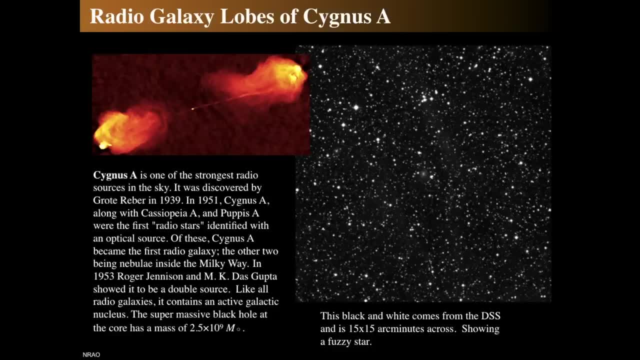 half a million light years or many half a million light years across. so it was discovered in 1939 by grotto rubber at grotti reiber and in 1951 as a bright, strong radio source. is it actually one of the strongest? and in 1951, along with cassiopeia a and pupa say were defined as radio stars as 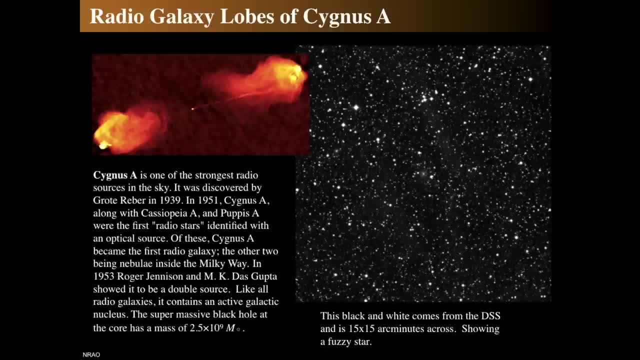 people were looking at. so people didn't know. you know, we first point radio telescopes in the sky. you just say, what's that called? some bright point like object, call it a radio star, okay, great. and so they were identified with, with optical sources, and so they were called radio stars. cygnus a is a radio galaxy and the other two, cassiopeia and 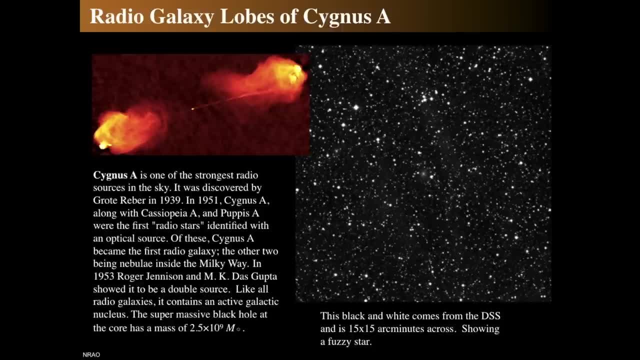 pupa say are are nebulae, with cassiopeia being that supernova run that we talked a while back about um and in 1953, just a few years later, jenison and tascoopta showed it to be a double telescope. everybody's saying, wow, this is neat, let's go look at it with radio telescopes and all. 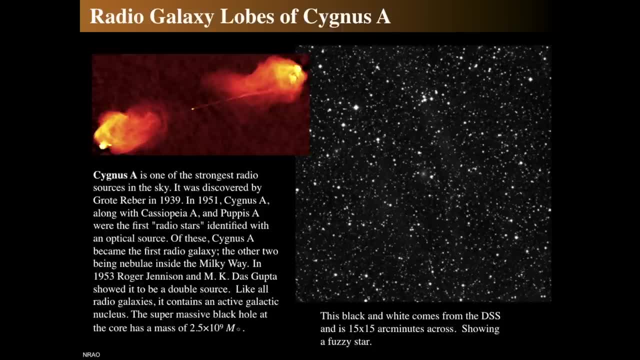 radio. galaxies, especially this one, have a huge, huge, huge active galaxy nucleus in the core and there is a super massive black hole about almost two and a half billion times the mass of the sun and the upper. that's the image in red. because of radio you have to kind of give it levels, that's. 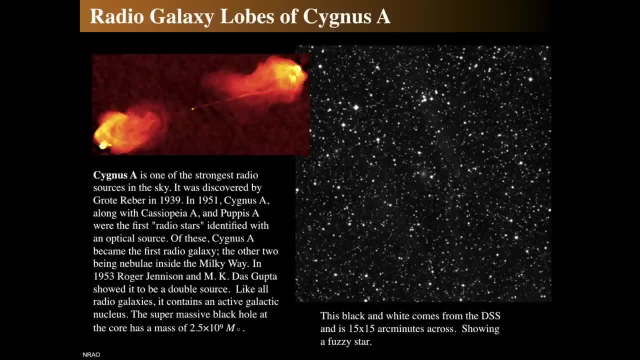 was taken by the very large array in the nrio national radio astronomy observatory and on the right hand side. what i did is i found this in the digital the radio telescope and i found this in the digital sky survey at space telescope science institute and made a pic and grabbed it by the 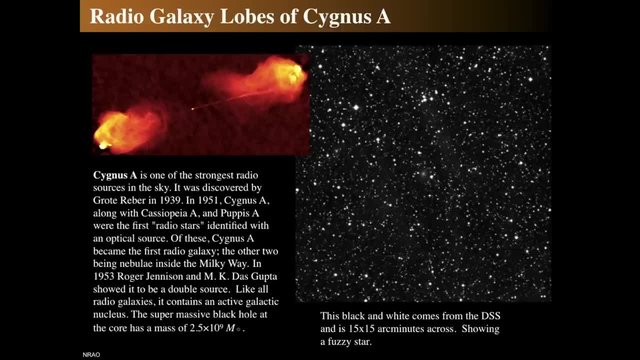 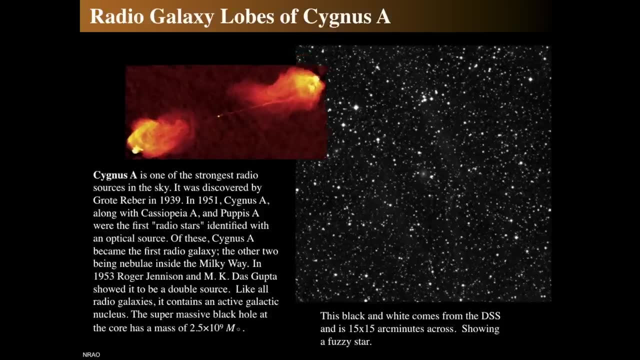 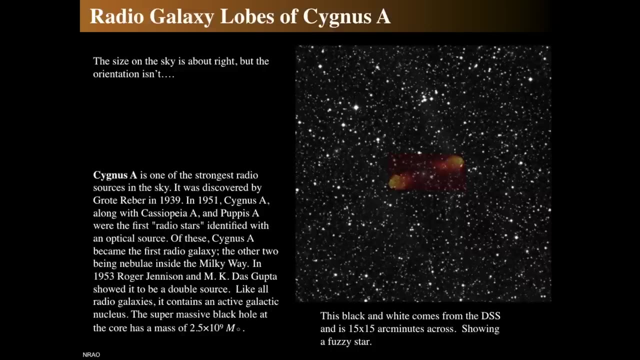 15 by 15 arc minutes to show what the region of the sky looks like in visible light. and this is the red image. but now what i'm going to do is i'm going to shrink it down and show you where it kind of appears on the sky. so that's roughly what it would look like if you could see it. it's, i don't. 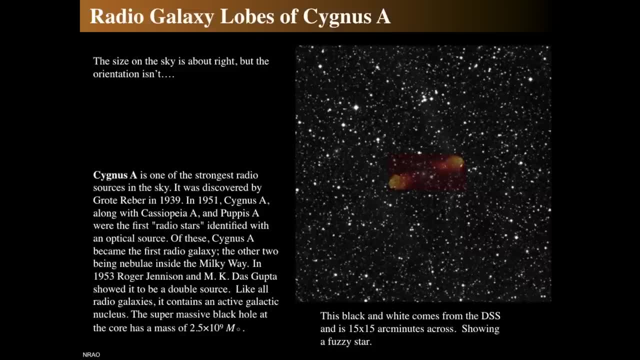 think the orientation's right. i think i got that wrong. but the point is is that it's kind of big, it's really bright. the galaxy itself can be seen and visible light, but the lobes cannot be seen in visible light. they can only be seen in radio and it's. 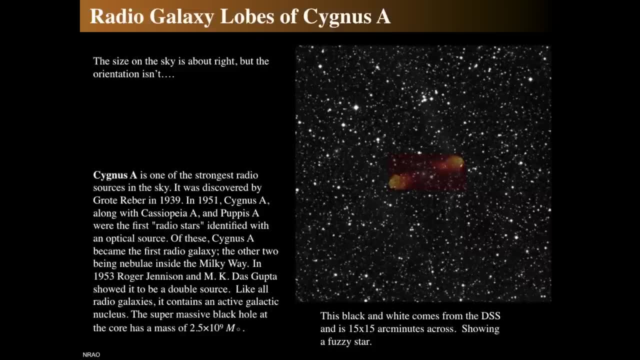 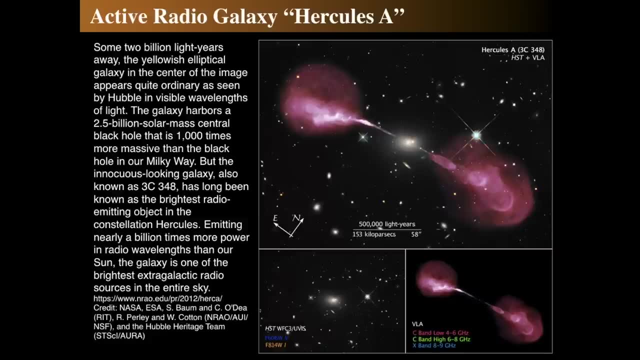 one of the strongest radio sources in the sky, at a half a billion light years away. another extraordinary, uh, extraordinarily bright one, is the hercules, a radio galaxy, and it was taken. the pinkish glow was taken by the very large array at three different bands and they mixed it together. 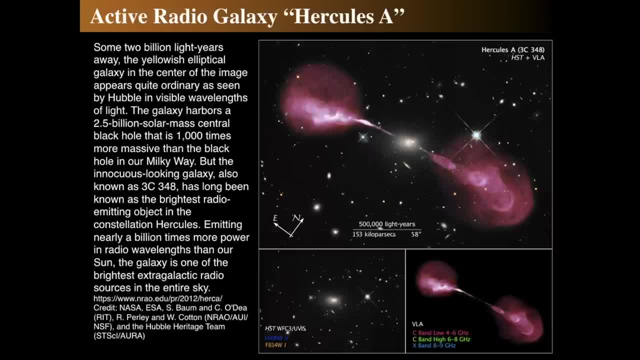 to form a red, green, blue and made some good images. and then the optical is the radio galaxy from the hubble space telescope wide field camera 3 and uviz. so this thing is almost two billion light years away and it's on, centered on a supermassive elliptical galaxy, um, and there's a 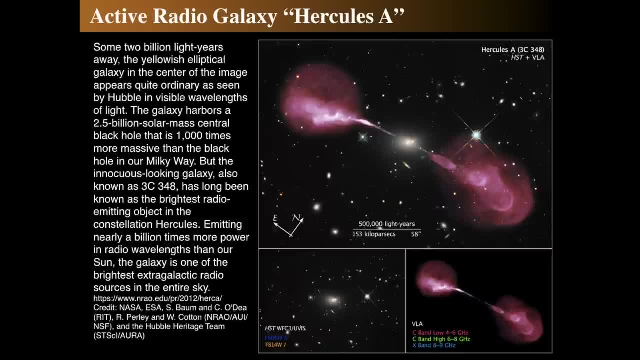 hugely bright galaxy in there. it's a two and a half billion solar masses and much bigger than the one that's in the center of the milky way, and what we find is that it kind of doesn't look like much invisible light, as you can see in the lower left hand image, but it's also. but since it's. 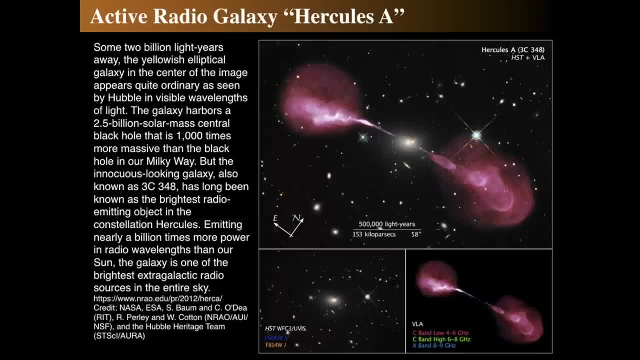 the brightest radio emitting object in the constellation, hercules. it's kind of crazy that this thing is, you know, half a billion light, two billion light years away, and it's even at that distance. it's a mil over a three, almost two million light years across from low edge of. 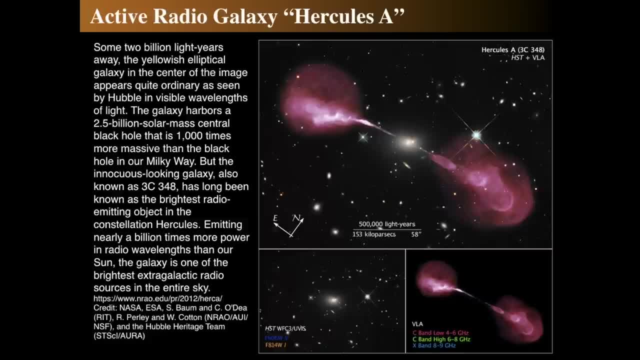 lobe to edge of lobe. so something is making these jets, something is making the jets, something is keeping it collimated for almost a million light years, at least a half a million light years, and then the radio emission then gets deposited out there and then it still glows in radio light. 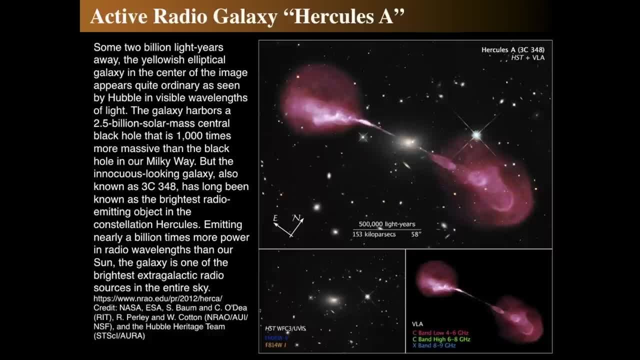 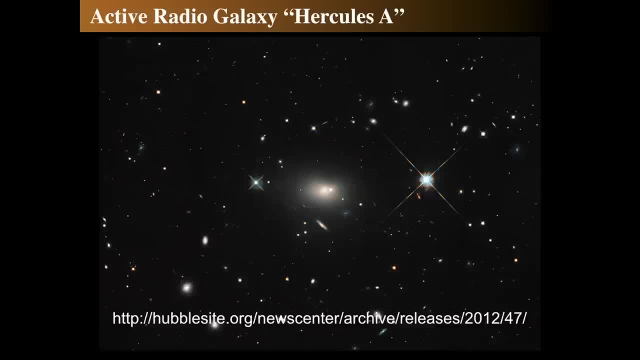 so the question then becomes: what exactly is making that radio emission and how does it stay in this jet-like format? and that's a big, big, big big puzzle. so there's the optical image of the visible image of hercules a and there is the hubble, and then there's the vla image overlaid. 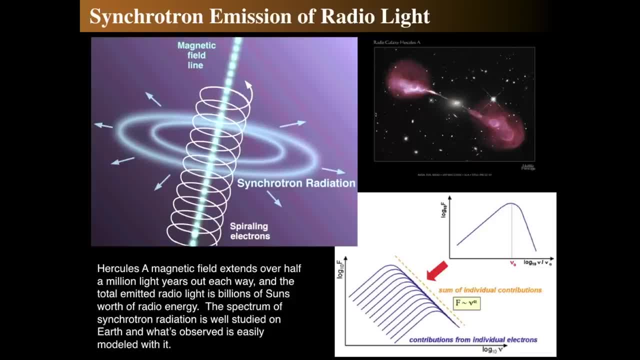 on top of that, and this is a hubble heritage image. well, what exactly is it? so it's? it's supposed- because it's radio light, so it has to be very low energy radio light- that there's a strong, strong, strong magnetic field. and that magnetic field is uh, it is actually causing electrons to spiral. 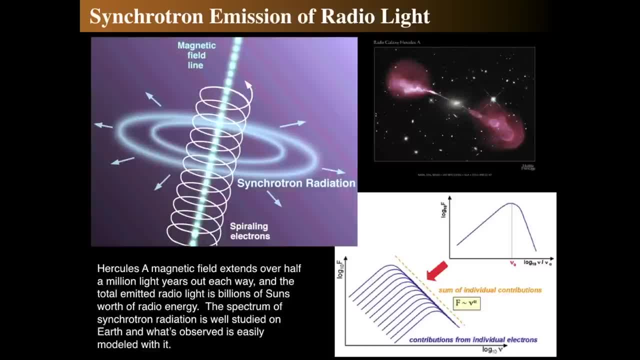 around. and that's what an electron will do in a magnetic field. if it has any motion, it'll kind of start to go around the magnetic field lines. it'll form a curlicue. now, if it's moving really, really fast, then what will happen is it'll form a helix and it'll 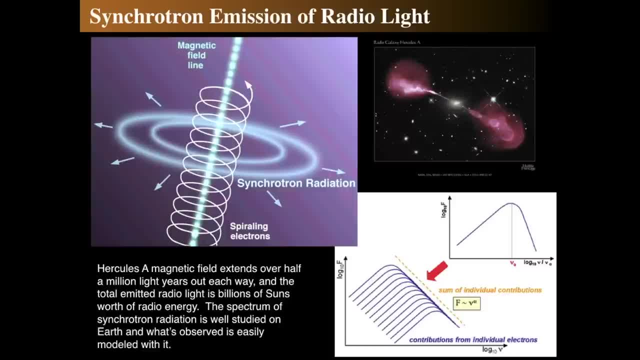 scoot around and if it's traveling at almost the speed of light, it has a specific kind of spectrum. a single photon, a single electron. uh will make a spectrum of light in radio light, like the hump that we see in the lower right inset, which is a single contribution from a single electron. 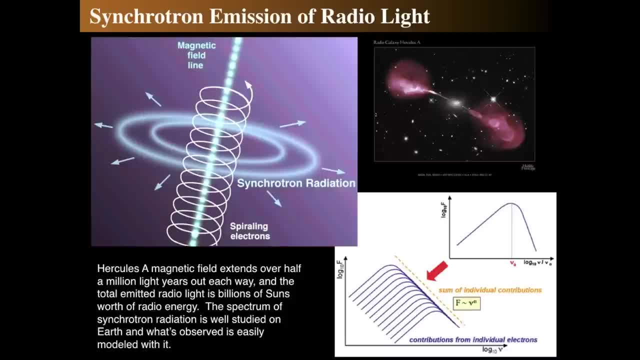 traveling at nearly the speed of light in a very strong magnetic field, or at least in any magnetic field, and some of the electrons are going to be traveling at a very strong magnetic field, are more energetic than others, and so, as they travel along the magnetic field lines, each one, 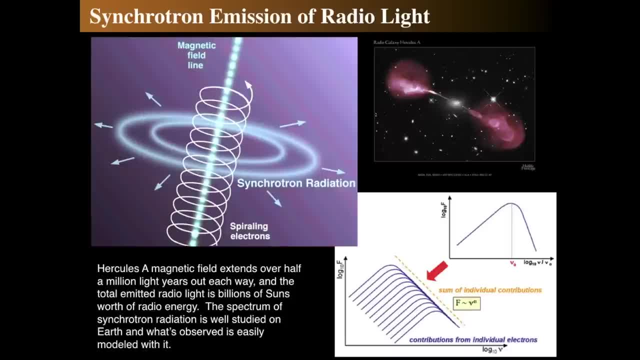 of those electrons each emits one of those kind of humpy sort of spectrum. so if you add up all the contribution from all of those individual electrons you get what the red arrow is pointing to, which is that dashed yellow line which kind of looks like the merging of all of those spectrum. 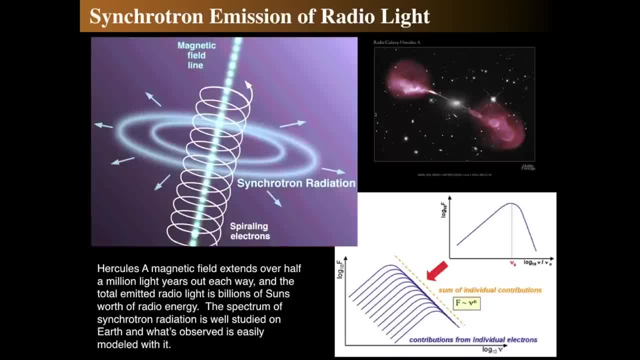 so you get what's what's called a power law spectrum, and that power law spectrum looks completely different from the power law spectrum of the electromagnetic field, and that's what we're going to talk about in a little bit more detail, in a little bit more detail, in a little bit more detail. 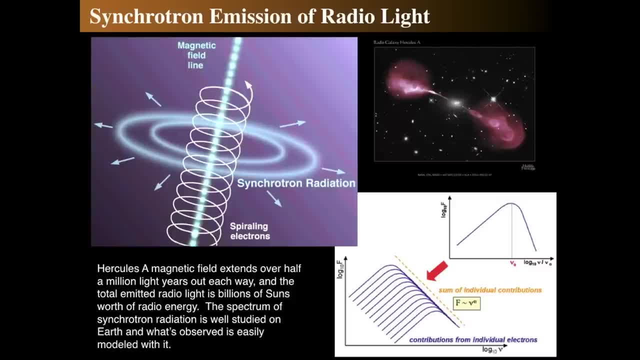 than say a black body spectrum, like we saw coming from stars. there's no absorption lines in synchrotron radiation, it's just this flat, flat, flat feature. so well we know about synchrotron radiation because of studies in in uh, in particle colliders, as well as nuclear physics studies. so 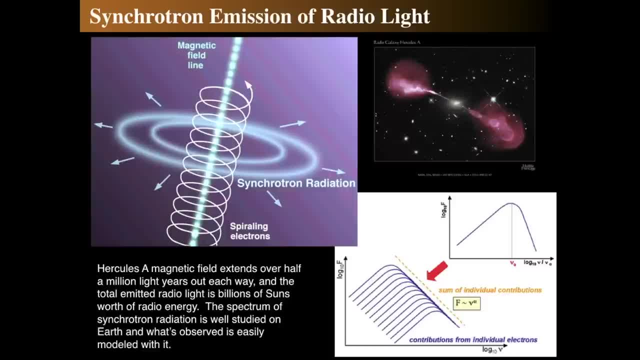 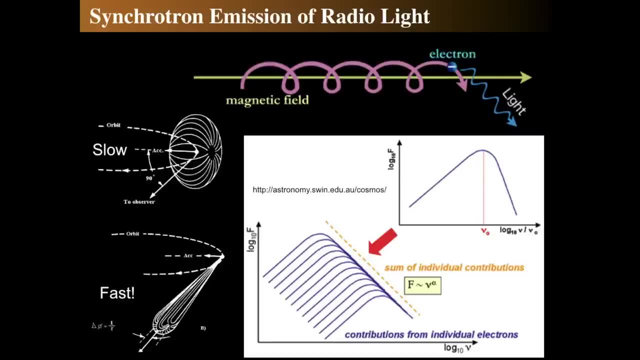 this has been. this process is well understood and it's interesting to be found in these radio galaxies. so here's another diagram to show it. and we see the electrons zipping around in the magnetic field and as it goes around and around and around, it emits light. and as it emits light, it 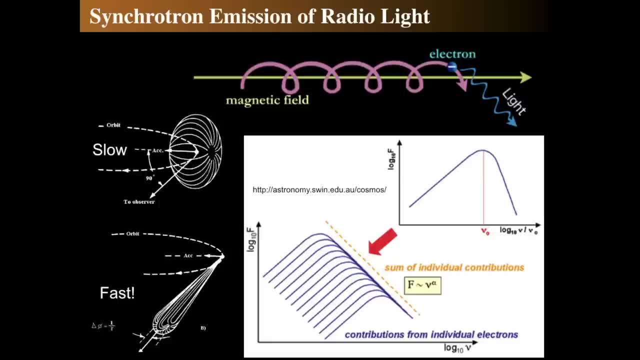 loses energy and therefore goes a little bit slower. so we also see, then, the the image of the sum of all of these things, and i grabbed. i grabbed this image from swinburne edu so you can go take a look at this. this is online on their website. now, on the left hand side, i kind of grabbed this other. 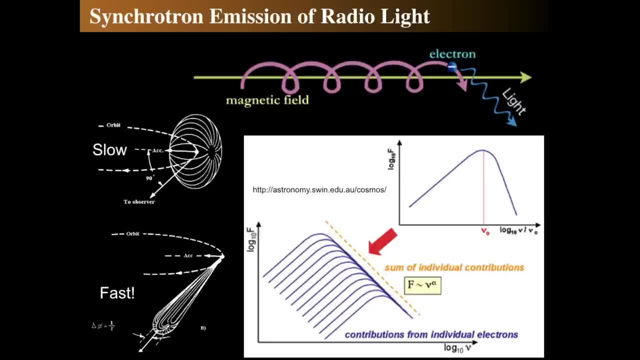 thing from wikipedia kind of try to show what i mean and why we think, why this is a special kind of spectrum. now, on the left hand side, i kind of grabbed this other thing from wikipedia kind of: if the electron is spiraling slowly, meaning you know kind of fast for normal people like it'd be, 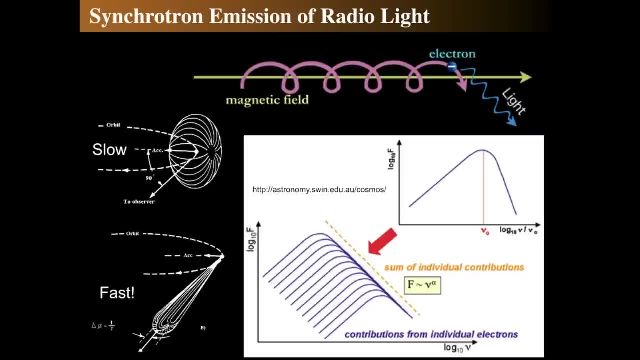 going faster than a person can go, but if it's kind of spinning slowly, not at nearly the speed of light, the emission that an electron would make because it is accelerating, because it's going in a circle. as it goes in a circle in a magnetic field, it will emit light and it will lose energy. 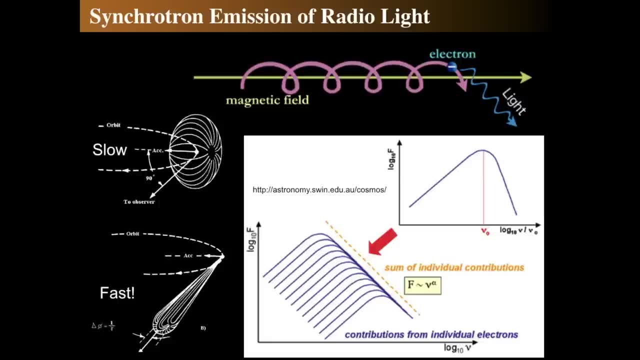 and that light emission pattern is shown in that kind of donut-y sort of bagel thing that we see. and that's the way the light spreads out from the electron as it slowly goes around a man in if it's moving slowly and moving an electric field or in a magnetic field. but now, if you take the same 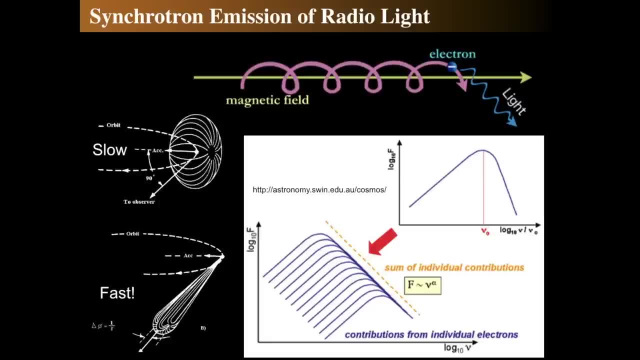 magnetic field and accelerate the electron up to nearly the speed of light, you get what are called relativistic beaming effects, where all of the light gets beamed in one direction, so the direction that the, the electron is going. so that chain, that that shape of the emission, as well as the 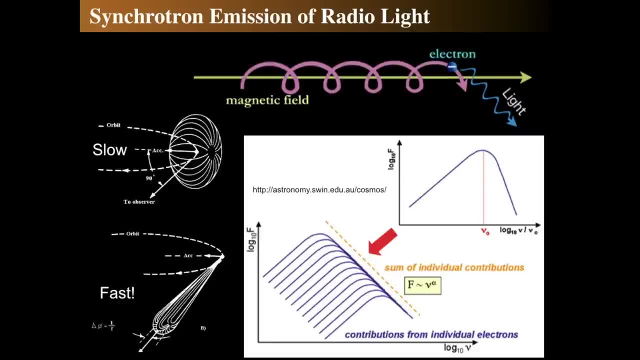 spectrum as well, dictates how the spectrum will look and that's what we see and that helps to this understanding of how it works and how the emission actually works with the light gives us an understanding of how we might get to the upper right hand sort of individual electron. 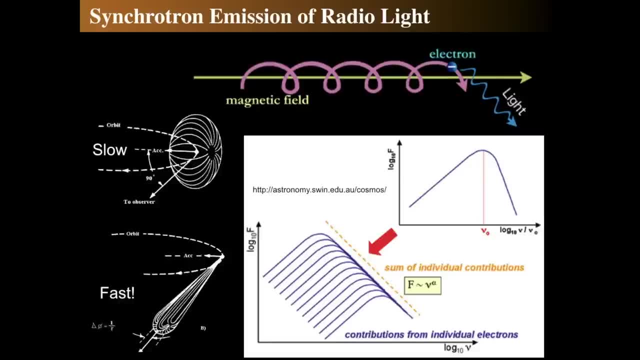 thing, but this is called relativistic beaming, and as the electron spins faster and faster around, actually it goes very fast and loses just the tiniest amount of energy because it's radio light. it's got a huge amount of energy on its own but it emits that light and gets lower and lower energy. but as they all emit in this particular way, 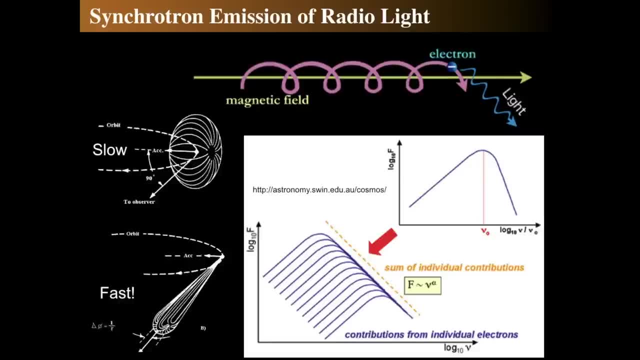 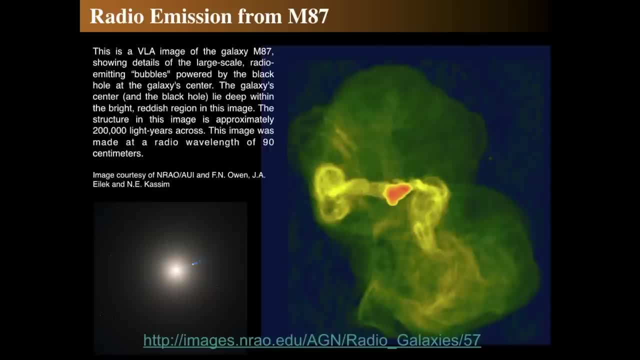 according to this model, you get the sum of all the contributions, and that model is also borne out by looking at nuclear physics labs. all right, so given that that's how these things kind of make their emission, let's look at some of the zoo of crazy things that we see out there in the nearby. 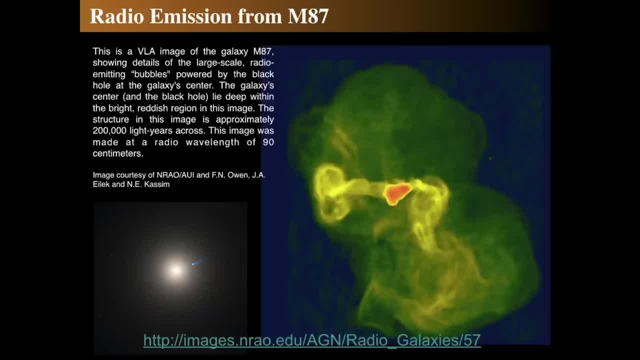 uh, virgo cluster, the galaxy m87, which is an enormous, enormous, supermassive giant, elliptical in the virgo cluster of galaxies, about 600 000, about 60 mil, 70 million light-years away roughly, and what we see is that there's these enormous. the lower left-hand image is an optical light image, but on the right-hand 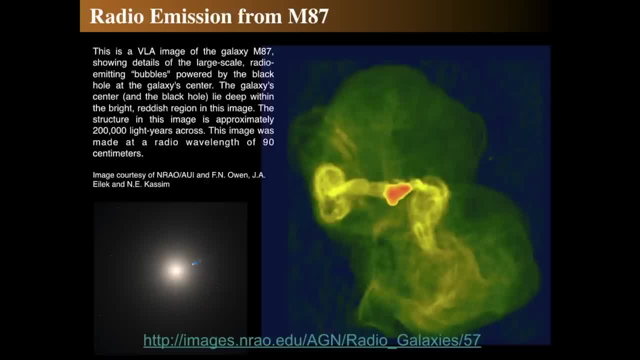 side is a visa, is a is a radio image of the same galaxy. so this is a very strange thing that they're completely different. there's these puffy things around it, there's these weird shapes. i don't know exactly how they superimpose, but the well this str, the structure on the right, is much, much, much different. 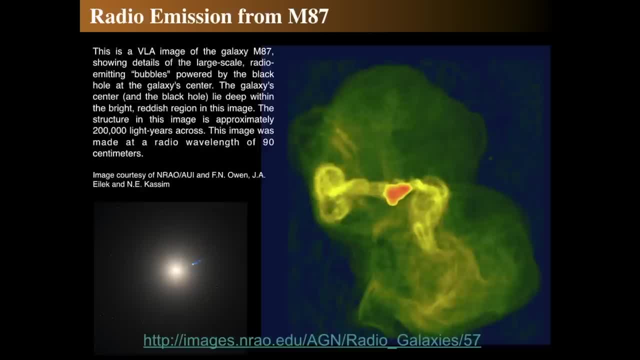 but the well. this str. the structure on the right is much, much, much different, much larger than the Milky Way At 200,000 light years across. this thing is easily. the green puffy thing is easily twice as large as the entire Milky Way. 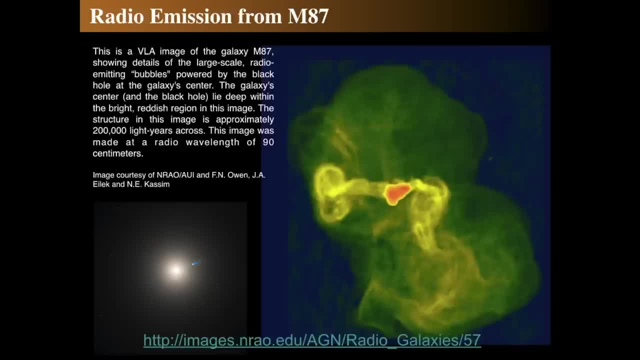 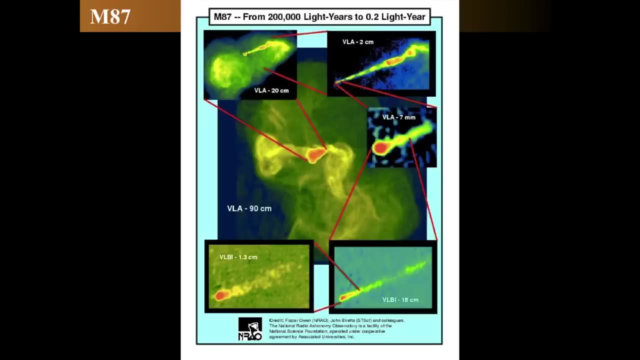 galaxy, But yet there's really bright core, compact regions, and then you see something that looks really jet-like, that's pushing stuff out. You can almost imagine that there's this jet of material being thrown out in two directions: One of them towards us and one of them away from us. So now here's a. 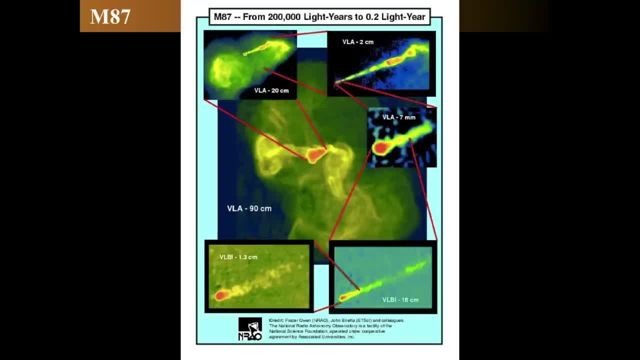 VLA study, a very large array by the National Radio Astronomy Observatory, done by Fraser Owen and John Battia at NRAO. And so we see that the VLA, looking at 20 centimeter radiation, shows that large jet-like structure in the center. So we 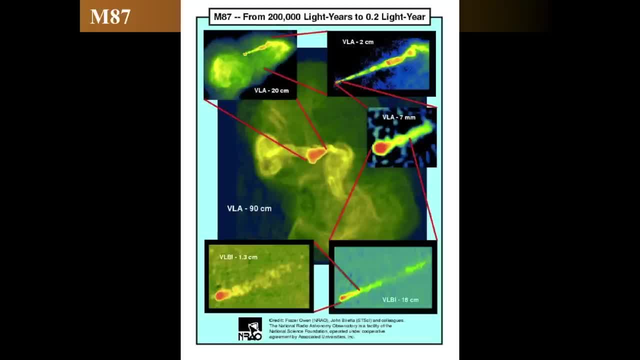 see the big, big, big map. Now we zoom in with the 20 centimeter VLA. We see a very tiny jet-like feature and the right-hand side is a jet and the left-hand side not so much. And then we zoom in closer and tighter with the 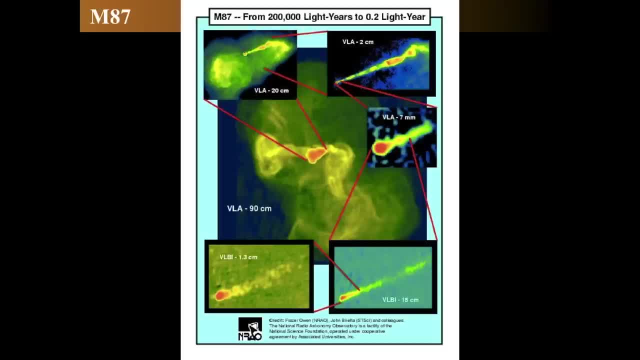 VLA At two centimeters and we see that the jet has deeper resolution. It has knots and wobbles and beads type of things. And then zoom in even tighter with seven millimeter wavelength radiation at the VLA and we can see almost the central. 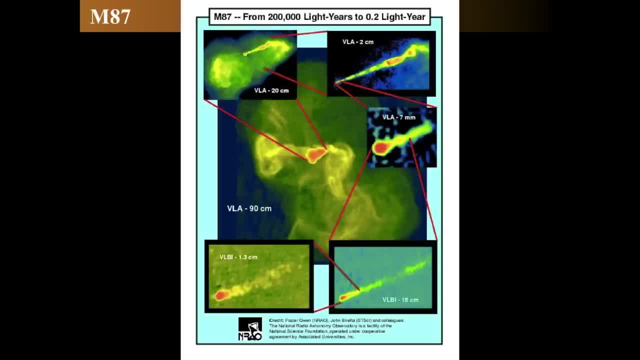 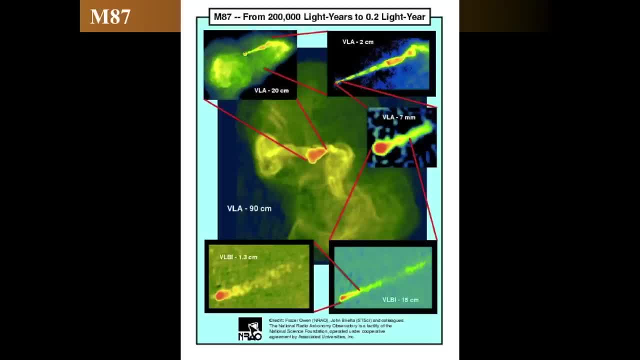 Plrale's, known for VLBI, which is very large baseline interferometry, which is not just the VLA telescope but numerous other radiotelescopes across the United States and across the world All combining their data together. they get higher resolution of that interior structure. The VLA is only so big. 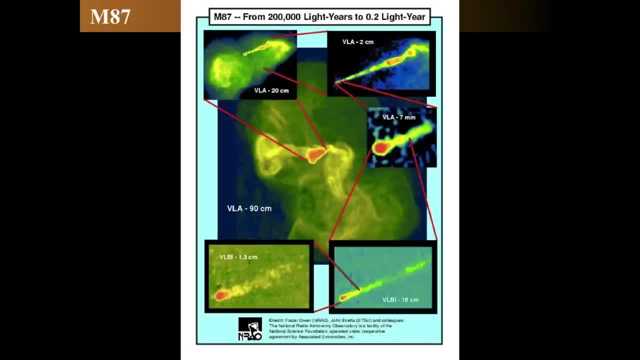 so the resolution gets poorer as you zoom in. But if you integrate a bunch of radiotelescopes together, such as the VLBI eye, then you get much higher resolution. But notice, as you zoom in, in, in, in, in, in. 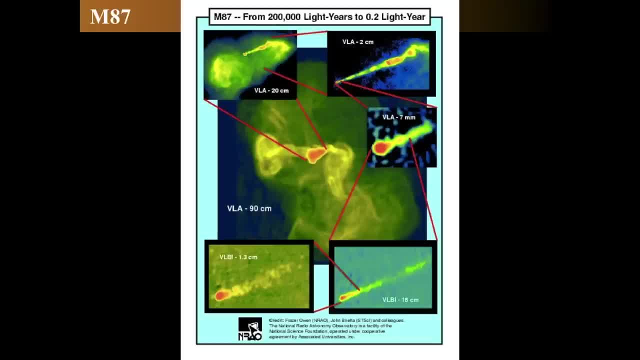 you still maintain a compact, tiny source. So the lower left-hand image shows something that's only a quarter of a light year across. What's a quarter like two-tenths of a light year. Two-tenths of a light year is a couple of light months right, Or even one light month. 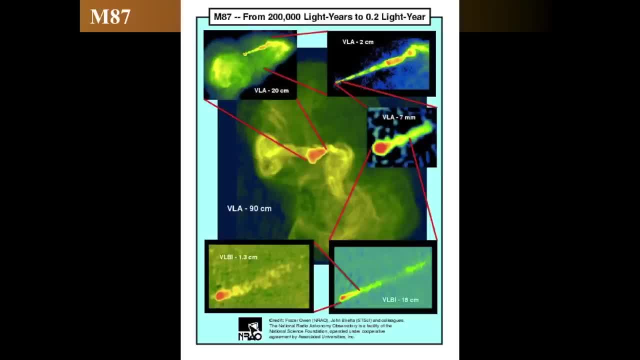 One light month is 30 light days. 30 light days is wow, that's a, that's pretty, that is remember the size that the Voyager has gone is almost a light day. So the image that you're looking at across, if you look at an individual pixel, a couple of pixels across this thing, 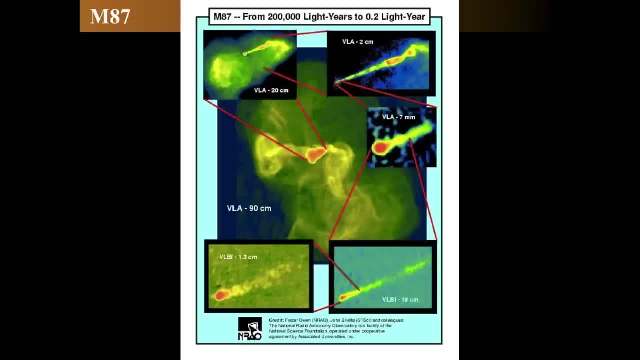 is what the Voyager has traveled since it was launched in 1977.. So a few pixels on this lower left-hand image is the distance Voyager has gone from Earth. So this is a really tiny, compact, extraordinarily bright object deep down in the core of M87.. 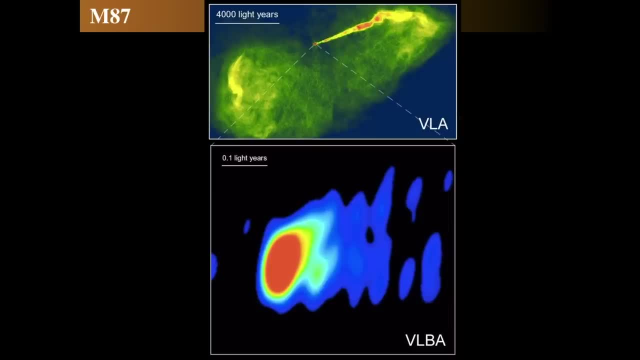 Once again, there it is. we're zooming in: VLA on the upper upper front and the VLBA very long baseline array showing the inner tenth of a light year- Remember a tenth of a light year- is on that orbit. 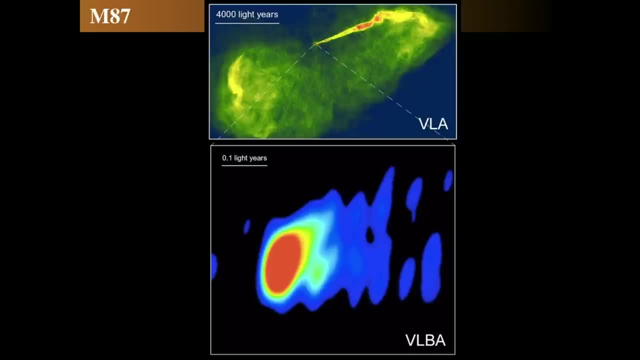 So we're looking at at objects or or resolution of a bright, compact radio source that is not that much bigger in terms of that bar. So that bar is is one. it's like one-tenth of that bar is what the Voyager has traveled since its launch. So actually, if the Voyager were a super-duper-duper, 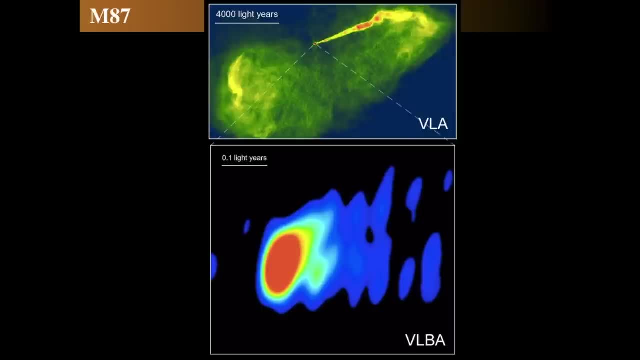 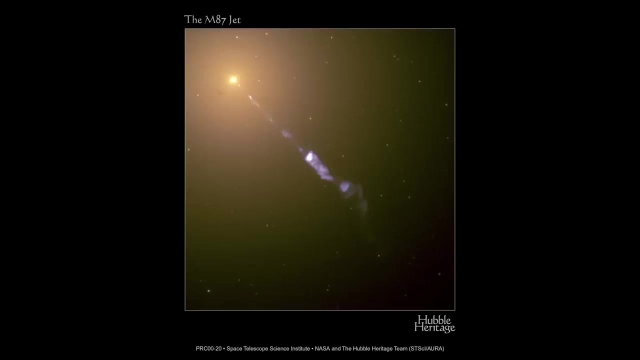 bright, point-like radio source. maybe it could be resolved, but it's not. it's not that bright. In any event, this is to just try to show you the size scale that we're looking at, something that can be easily measured in terms of solar system size, size scales. And there it is, with the Hubble image showing the jet. 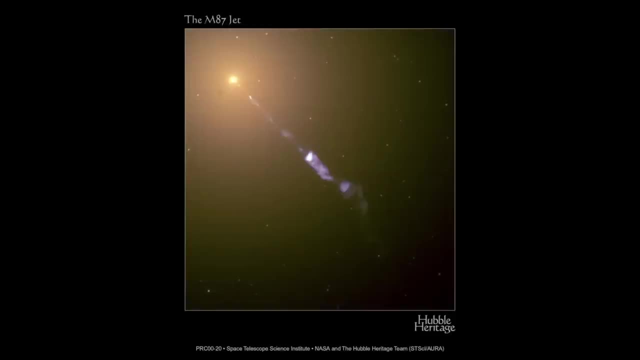 in visible, visible light. So there's something going on in radio, there's something going on there and we described that the radio emission comes from synchrotron radiation, that's coming from the spiraling of electrons in a strong magnetic field. Now you can get visible light. 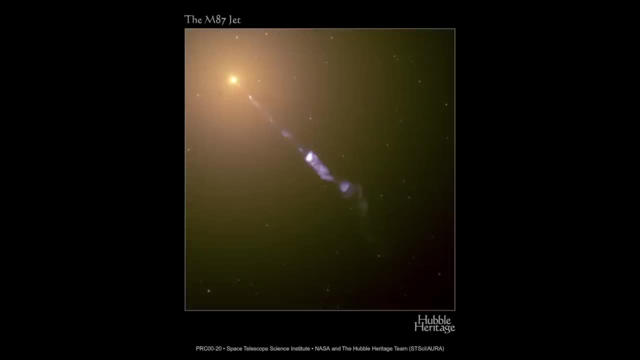 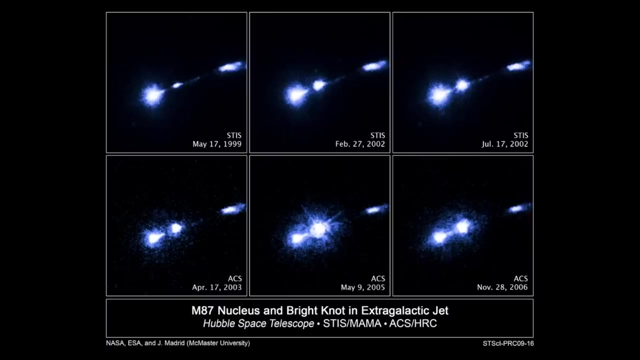 and you can get x-ray radiation from that as well, and that's what we're seeing here in this, this jet coming from the center of M87.. And there we see M87 using the Hubble space telescope done by uh Jay Madrid at McMaster University, showing actual changes in the visible light of that bright. 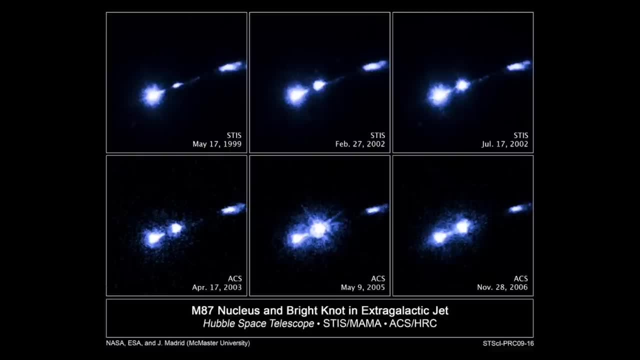 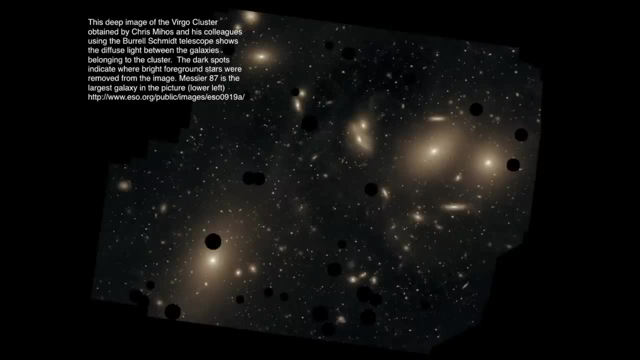 knot in the center of the, in the center of the galaxy of M87. And just for enjoyment, to get you an idea where the heck this thing is, the lower left is the is M87, the giant, supergiant mass of elliptical galaxy. it's in the Virgo cluster And we're seeing a super giant mass of elliptical galaxy. 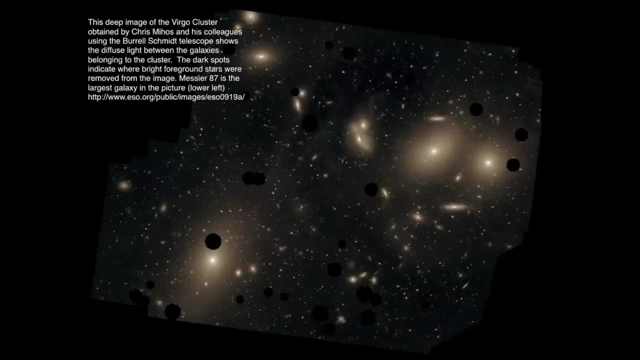 and we're seeing a cluster of galaxies here And this was taken by Chris Mijos and the colleagues at the Brunel-Schmidt Telescope And this was done with the European Southern Observatory And they took out all the foreground stars and that's why they've got those spots of bright. 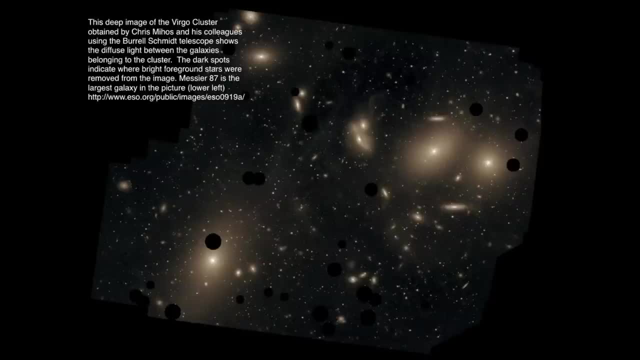 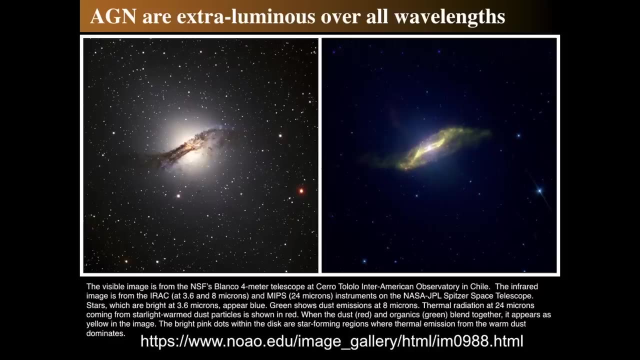 Because you know we just want to deal with the stuff that's actually the galaxies and not look at the stuff necessarily and not be distracted by things that are in the foreground in the Milky Way. All right, Another thing we can remember with active galactic nuclei is they're really luminous. 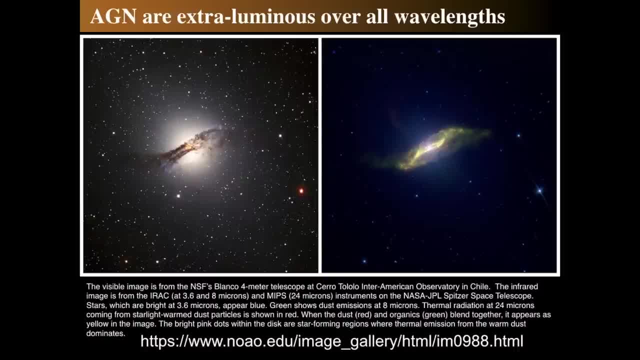 extraordinarily luminous over all wavelengths. And on the left again, we go back to our favorite, which is Centaurus A, which is one of the most interesting, which is one of it's a favorite target for active galactic nuclei studies. 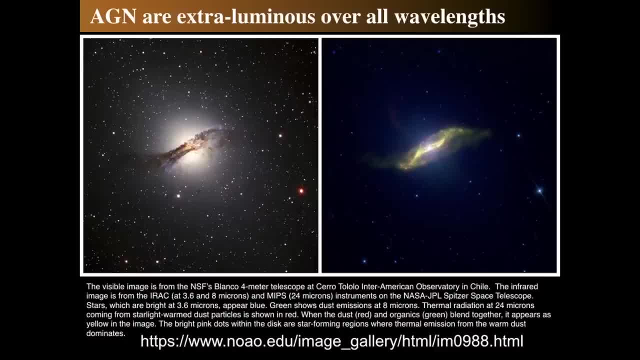 And on the left we see a visible light image taken by Sarah Tololo at the IAO in Chile, the Blanco 4 meter. But on the right-hand side was taken by the Spitzer Infrared Space Telescope run by NASA Jet Propulsion Laboratories. 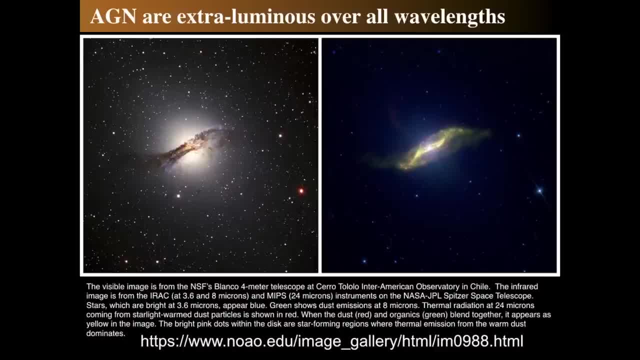 And so we have emission from that, From thermal emission, from that which is, we have dust and gas and thermal emission, but you can also still see dusty, gassy, distortions. It's extremely bright in the center And we also see that there's some sort of jet-like structure coming above and below. 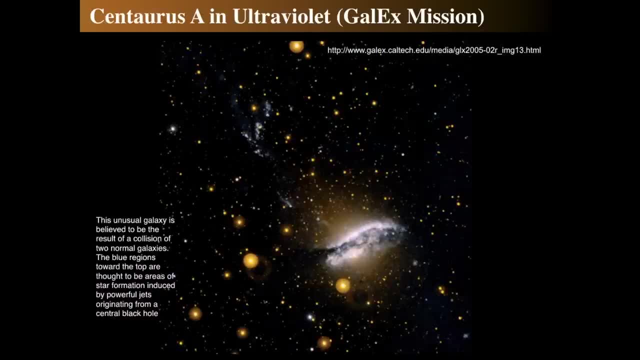 So there are extreme activity in infrared too, And if we look in ultraviolet- and this comes from the GALAX mission and there are some jets coming off of that And maybe even the jets that are coming off of that indicate star formation- 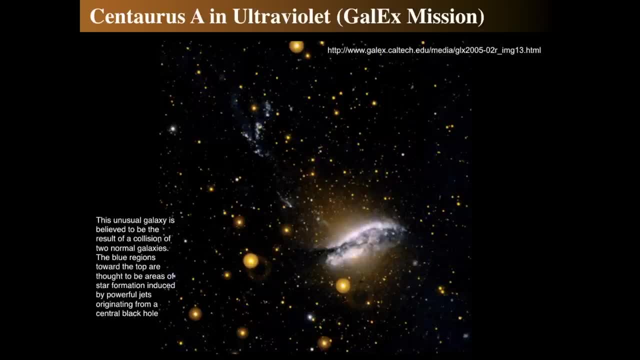 that's happening deep in those jets as a result of of collisional activity. That's one possibility, but perhaps it's just a synchrotron radiation again. But this is ultraviolet light, with the bluish-whitish light being higher energy ultraviolet. 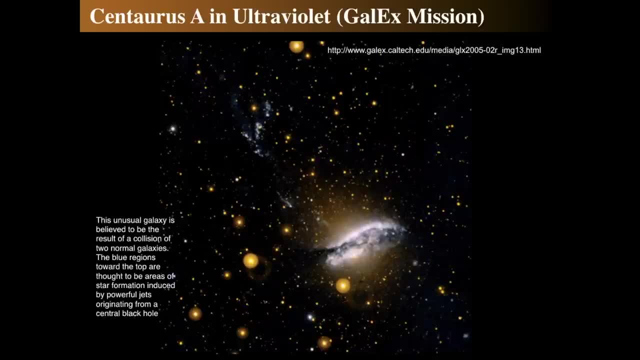 and the yellowish light being lower energy- ultraviolet- And so ultraviolet is interesting because you get these kind of circling structures and that's because of the nature of the detector itself, not because they're bigger objects. No, we're looking into those yellow spots. typically are stars. 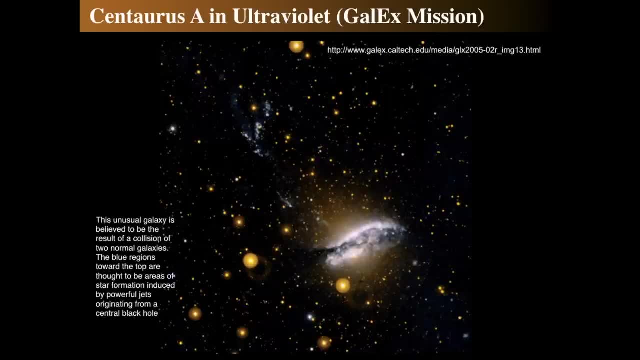 in our, in our galaxy, all right, But you also see there's a density around them, So that indicates there's some activity happening around Centaurus. A Notice: there's a cluster of those light yellow dots, So there's something happening as the two galaxies are colliding and making hot stars. 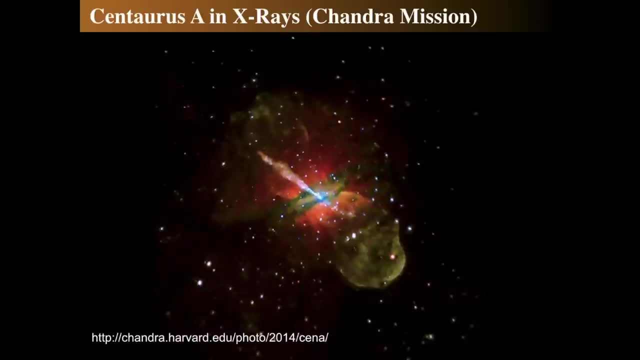 Again, we can look at the at Centaurus A and we see in X-ray light. this is from the Chandra X-ray Observatory, from from from one of their earlier studies, And we can see that the jet is formed from this, from from the. 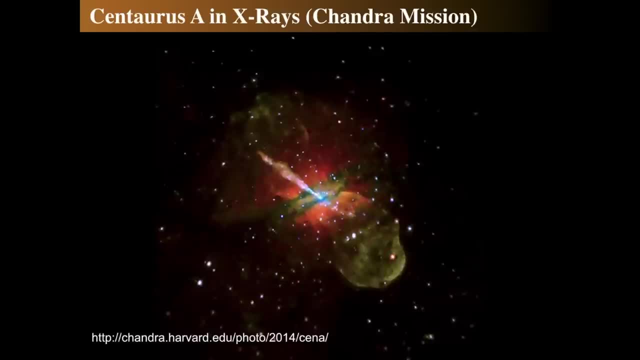 from the X-ray observatory From various processes in X-rays And we see the bubbles that also that are visible in radio light are also visible in X-rays. So Centaurus A has a completely different appearance in X-ray And we see an extraordinarily luminous hot object in the center. 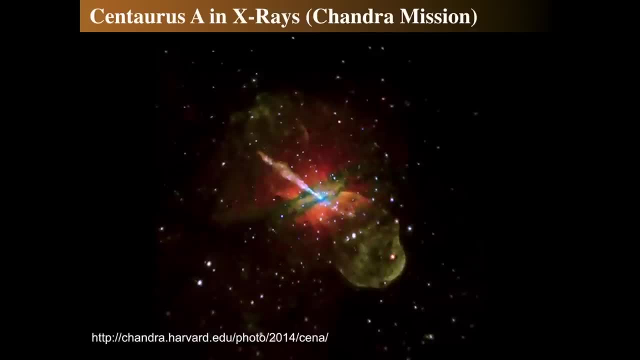 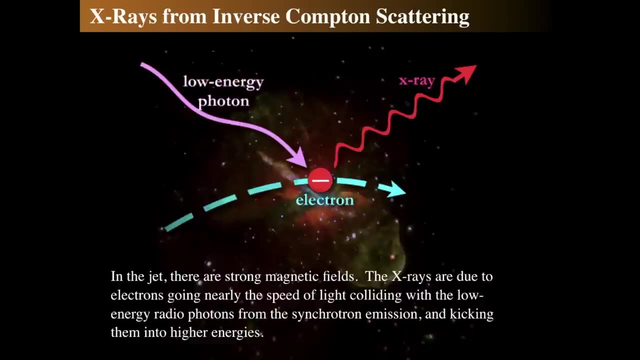 And the bluer the light in this image, the more energetic the X-rays we're looking at. So how do we get X-rays out of this? Well, one way is remember that there's electrons spiraling around it nearly the speed of light. 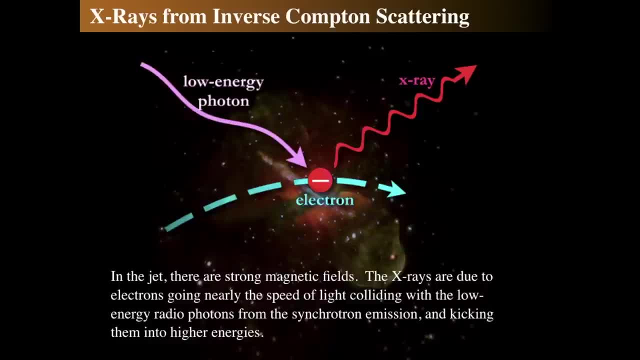 And they're emitted, And they're emitting radio light. What can happen is the radio light is a low energy photon. The electrons are moving really fast, And so they can collide with the photons and give some of their energy to the photon and bump it up to an X-ray. 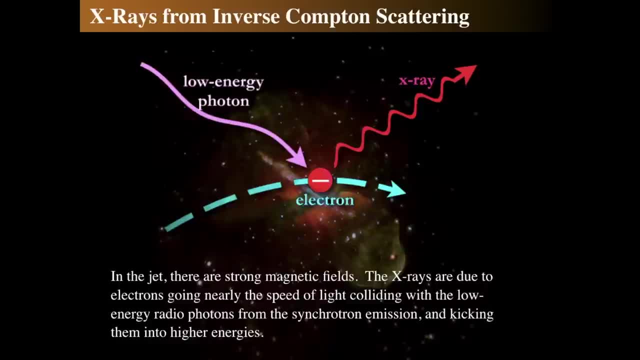 So the strong magnetic fields keep the electrons flying. Something's accelerating the electrons to nearly the speed of light and keeping them entrained inside of these, inside of these jets, And so we get X-ray emission from the radio light that they emit. So not only do they emit a radio light, they then billiard ball some of the light to get up to X-ray emission. 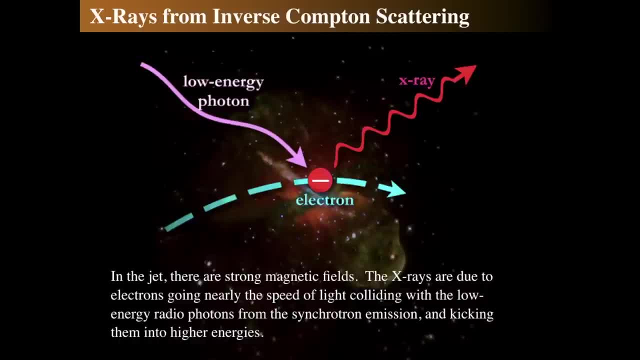 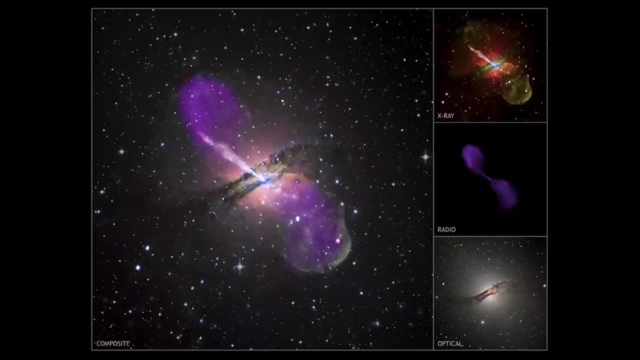 And we call that inverse Compton scattering. So it kicks them up into high energy as they interact and gives them more energy, And that's where those jets appear. That's what most of this emission that you see comes from. So here's a series of images, a composite of radio imaging, X-ray imaging and optical imaging from Chandra, VLA and the Hubble Space Telescope, as well as others. 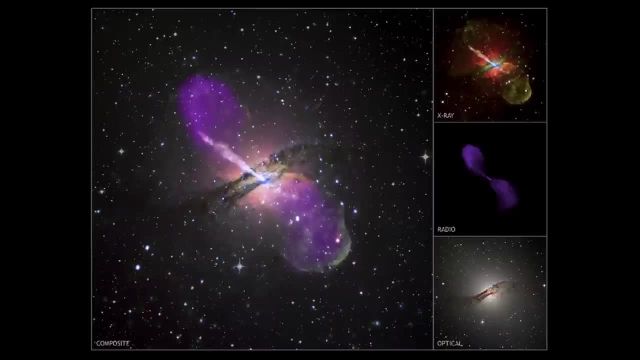 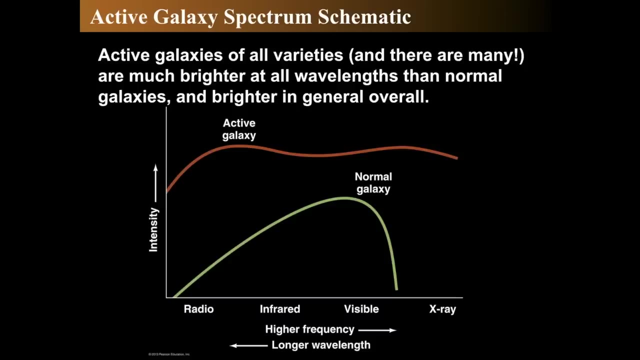 To put it all together to show you what an active galaxy in the nearby solar neighborhood is like. We're not solar, We're talking about 14 million light years away, So we've alluded to the idea that these things are bright at every wavelength. 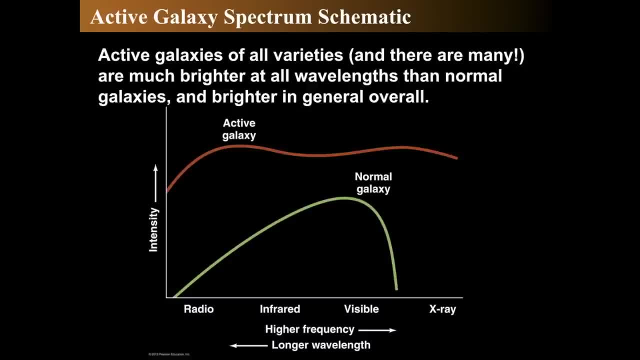 And active galaxies are. So a normal galaxy seems to be usually a collection of stars and gas and dust. So the lower curve shows a typical normal galaxy which would have a dim radio infrared invisible, But it's mostly an addition of a whole bunch of stars together 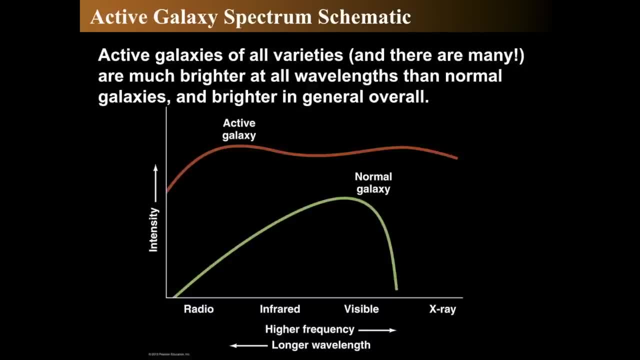 And we're kind of smoothing things out to make it easier to understand. but that's the basic idea. But in an active galaxy there's enormous radio emission, there's enormous infrared emission, there's enormous visible light and much, much greater X-ray emission than in a normal galaxy. 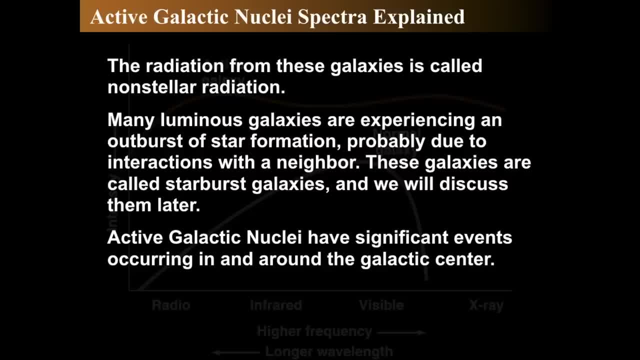 Normal galaxies don't tend to glow in X-rays, So the radiation from these galaxies is what we call non-stellar, meaning it doesn't come from stars Just like I described. we have electrons zipping around making radio light, and then they kick it up to X-rays. 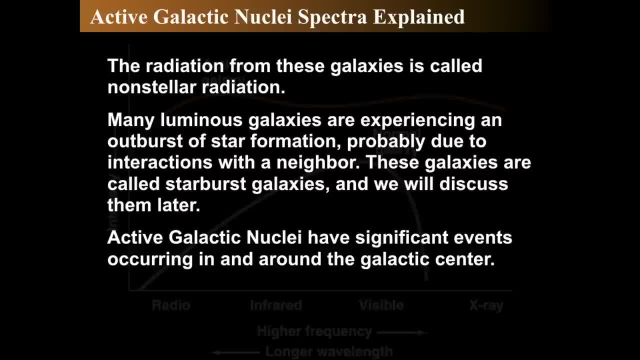 So this is non-stellar. This is not a thermal process that happens in stars. This is happening in magnetic fields, as things are moving at nearly the speed of light And something's actually accelerating these electrons and protons, or mostly electrons. It seems to be the dominant model to actually make all this light is high-speed electrons. 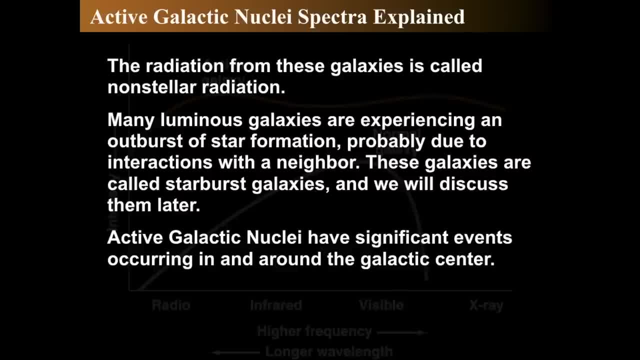 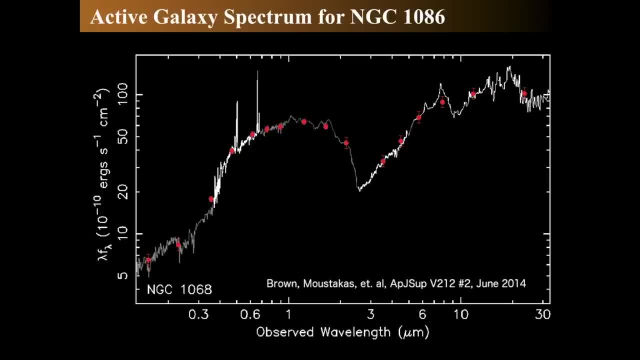 So something's happening deep in the galactic center to actually do that, So just to kind of really show a really high-resolution spectrum. So we go way back to Seifert's original paper, And this is by Brown and Moustakis again. 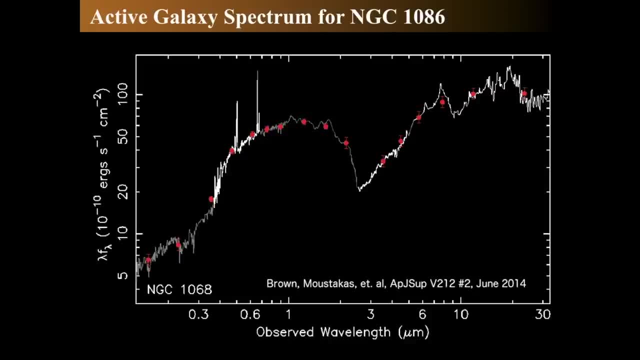 And this is from June of 2014,, where they took a large, large, large number of data and made what's called a spectral energy distribution, or SED: The entire spectrum of the galaxy, from very, very deep in the ultraviolet all the way to very long infrared. 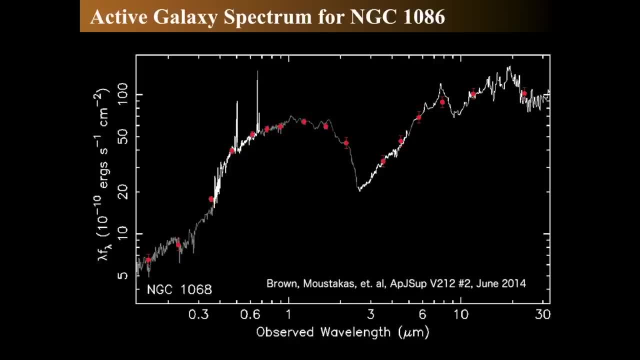 And so the visible light wavelengths are only in between about, say, 4000 and 0.4 and 0.7.. And 0.7 on this graph at the short end of the wavelength in microns. But then everything to the right is in infrared and everything to the left is ultraviolet, is out into the ultraviolet. 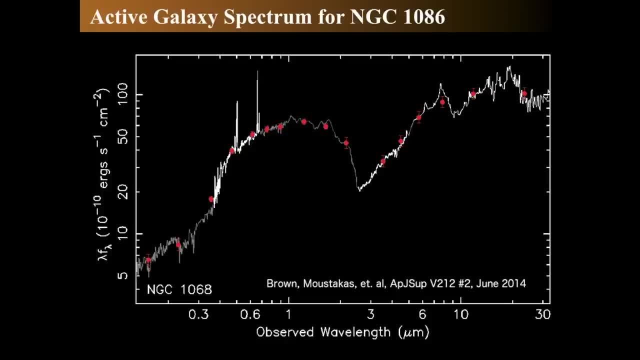 We don't go to the X-rays in this particular image. That's unfortunate, But we're seeing that this is very different than most normal galaxies because of the excess brightness in infrared, as well as the enormously bright hydrogen emission lines which you can see in emission here. 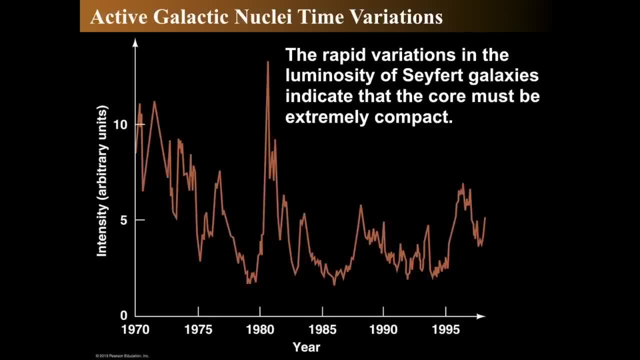 Now we're going to talk about the nature of the raptor. So rapid variations. Seaford galaxies vary really rapidly And this is kind of a schematic diagram by which they- well, what do we mean? They've got to get bright and dim by two or three or five times over the course of a few days or a couple of years. 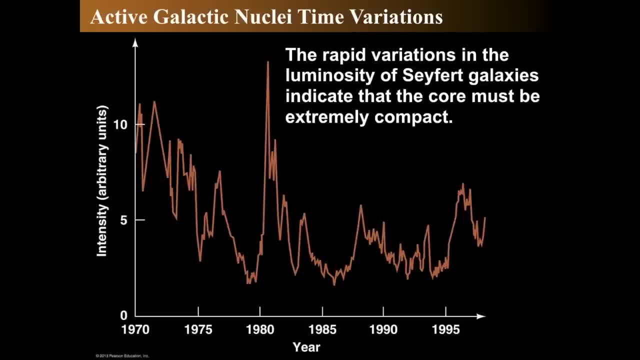 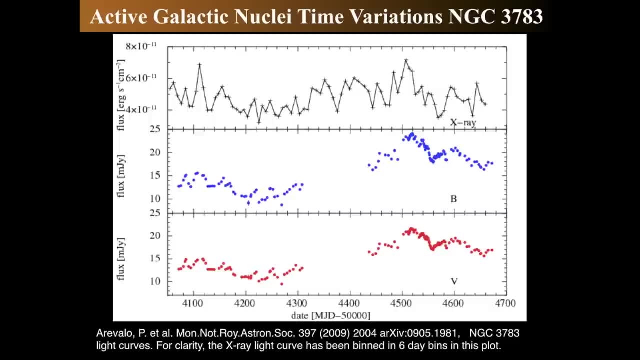 And they can actually be measured year to year, day to day, month to month and sometimes even day to day that they have their time variations. So what do we mean by that? This was a study done by Aravalo et al. 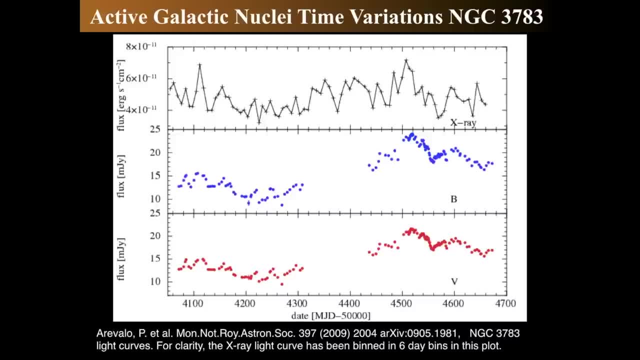 And they published it in Monthly Notices in 2009.. And this is an active galaxy, Active galactic nucleus: NGC 3783.. And they took three different sets of measurements- one in X-ray and one in Johnson B filter and Johnson V filter- over a number of days. 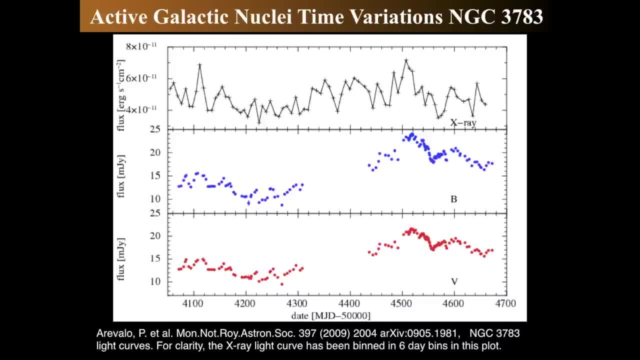 And, as we can see, there are lots of variations And this is varying. Just the nucleus is varying in brightness in X-ray, quite rapidly, as well as in the Johnson B, which is a visual filter, the blue end of the spectrum, and Johnson V, which is smack in the middle of the optical 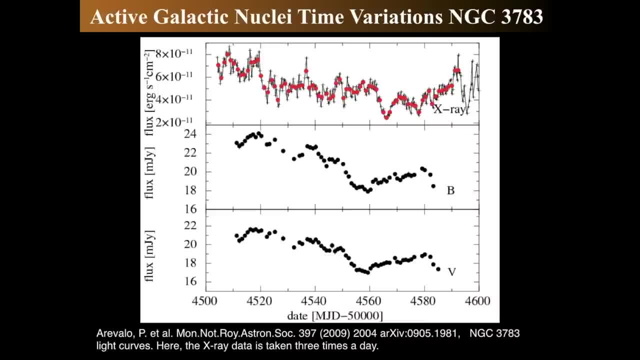 So then we actually zoom in on a very short period of time when they actually when they were able to take measurements up to three times a day, especially for the X-ray data, And they found that there's very high variability for the B and V spectra, B and V photometry of just the nucleus of this galaxy. 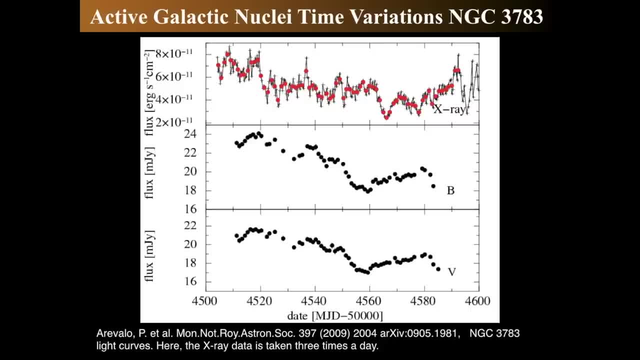 So this is a relatively nearby one, or else you wouldn't be able to get B and V photometry for it of this quality. But you can see that the X-ray variability can vary up to a factor of two Over the course of literally hours. 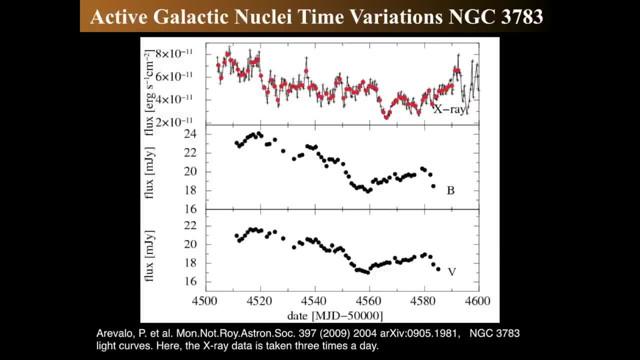 And the fact and the amount of that can come from the B and V in terms of. well, the word flux means how much energy you're getting per second into this, into your tiny little detector. Meaning ergs is a measure of energy: erg per second per square centimeter. 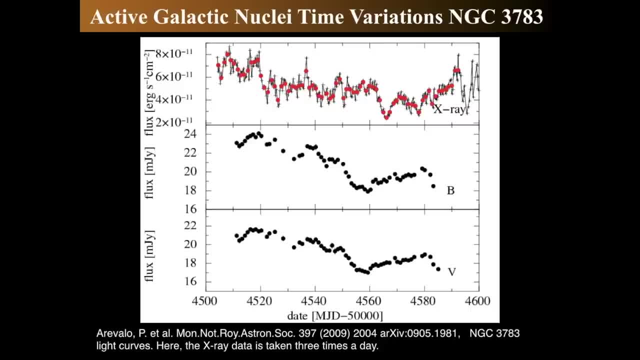 So if you had a square centimeter detector, you would get this many ergs per second, And an erg is a measurement of energy, just like a joule, So it's just in CGS units rather than SI. Okay, so we can see that there's extraordinary variability on the order of hours. 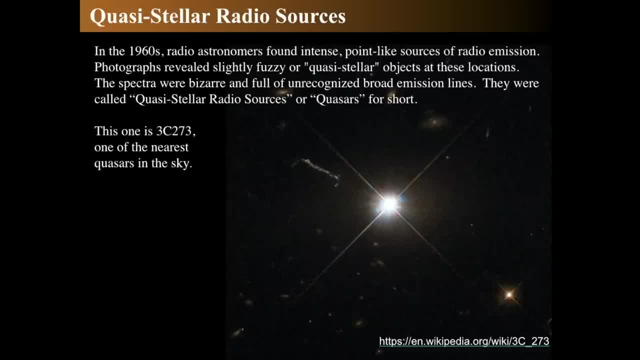 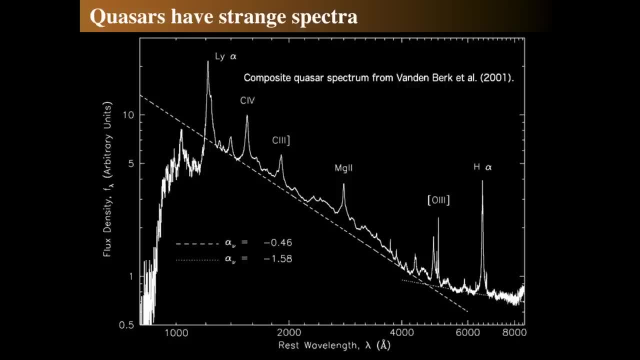 And then, when they looked at the photographs, they found there was a really fuzzy, tiny, fuzzy little star-like object that seemed to be like a star, And this is called a composite quasar spectrum. This was done by Van de Berck in 2001.. 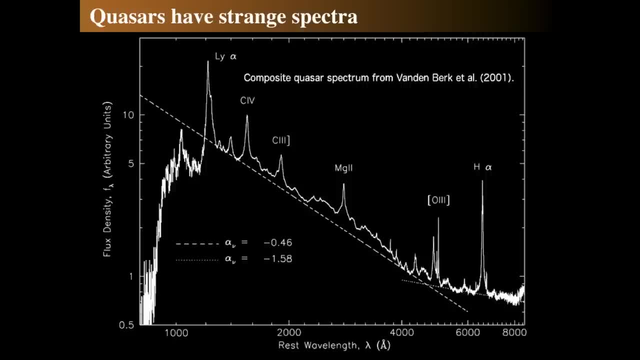 And what we see is that there's enormous, enormous ultraviolet emission at the Lyman-alpha line. That's for hydrogen, That's the Lyman-alpha. Then there's carbon…ionized carbon and magnesium-ionized, as well as ionized oxygen lines. 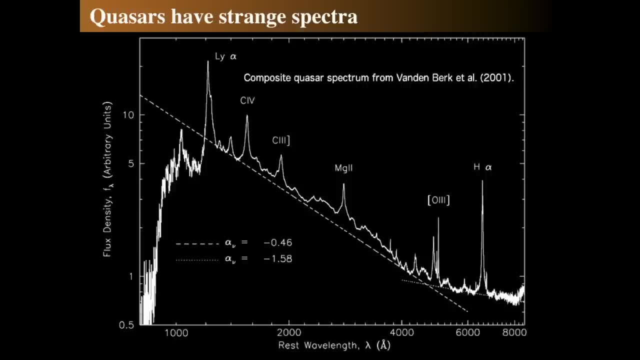 Hydrogen as well, is an extraordinary emission too. So we've got this amazing, strange sort of broad, broad emission lines, especially the Lyman-alpha line, which is insanely broad than anything else in the sky, and it has kind of a semi stellar sort of. 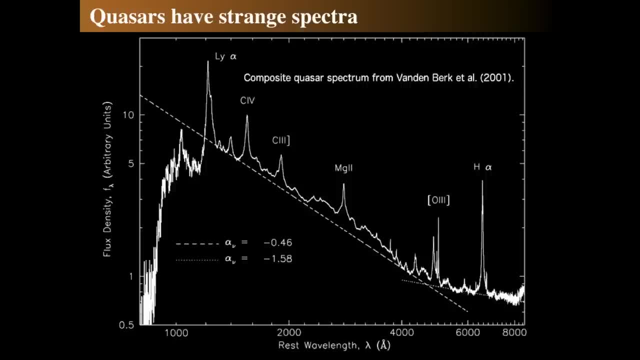 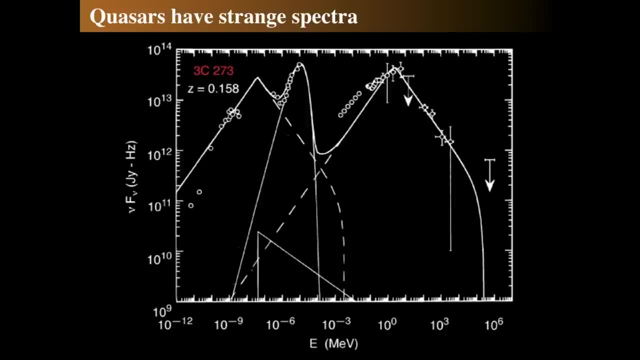 appearance because look at that shape. it's almost like a star, but there's something weird about that. on the left hand side, and here's this: the total wavelength spectrum across all wavelengths for 3c 273 and the circles are the actual data points and maybe there's some bars that go up and down to. 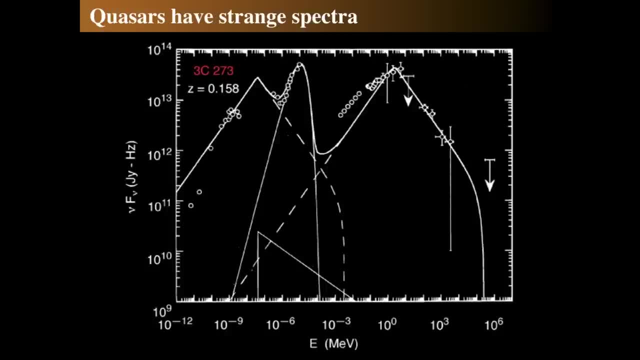 show you how well it's known. but on the far right hand side are extraordinarily energetic photons like x-rays and gamma rays and on the far left hand side are extraordinarily long wavelength photons like radio. but on that there's. so there's three kind of humps and there's like an additional sort of hump in the 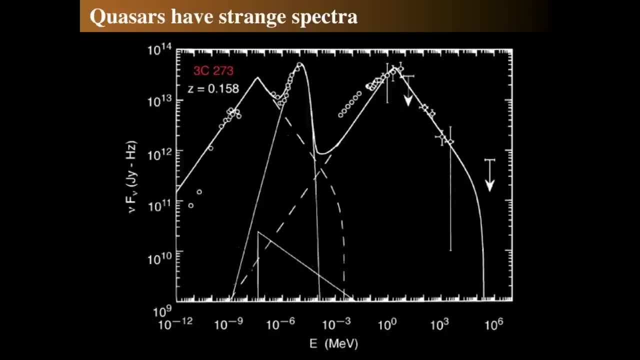 middle too. but let's actually look at the three tall humps: the one that looks kind of like in the middle, the middle hump that looks roundish. that's from thermal emission, or the sum of all the stars in the galaxy surrounding 3c 273. 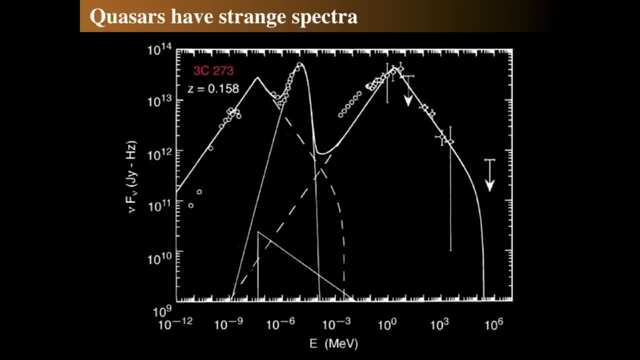 and so that's what the data points there show. on the left hand side is emission from radio, emission due to synchrotron radiation, and that's the long wavelength. stuff on the right hand side is x-ray and gamma ray emission that comes from synchrotron, that comes from the inverse. 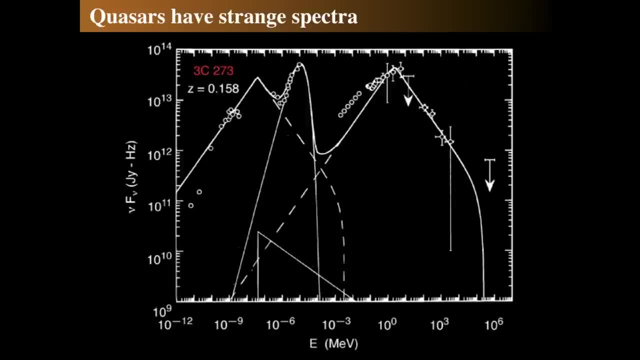 Compton scattering process that I described before, and so there's an enormous jet. there's three separate processes that give dominant radiation. so the idea that this kind of models the spectrum really well actually when you combine it together and the top line, is just kind of the best fit. 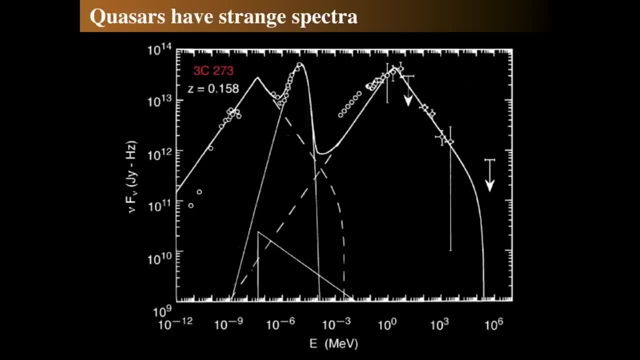 overlay. on top of the three underneath curves and the other one down below is another contribution which I forget exactly what it does. I think that might be dust emission. it's probably more like dust emission because of it kind of goes up and then drops off rather rapidly. all right, therefore. quasars are. 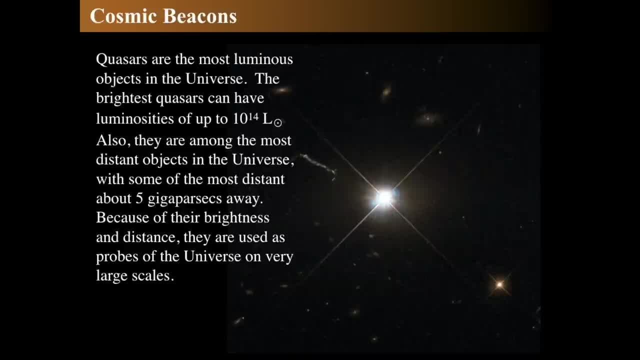 the most luminous objects in the universe. they can have up to something that's a hundred. that's a hundred, a hundred trillion times the luminosity of the Sun. a hundred trillion times the luminosity of the Sun. not billion, but a hundred trillion. remember, the luminosity of the Milky Way is about ten to as. 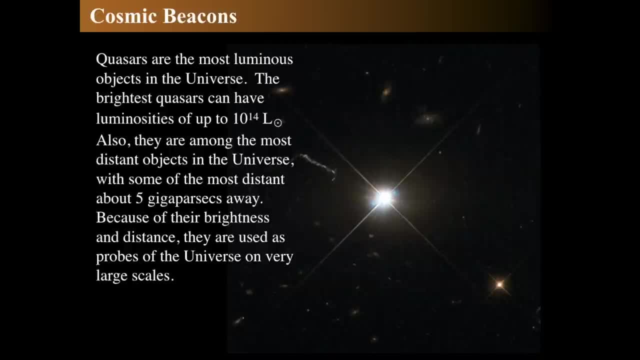 about a hundred billion, or ten and ten to nine, ten and ten to the eleventh solar luminosity. so this one object can have a thousand times the luminosity of the entire Milky Way, and most of the light from this is coming from the center of the object. this thing I've mistook. 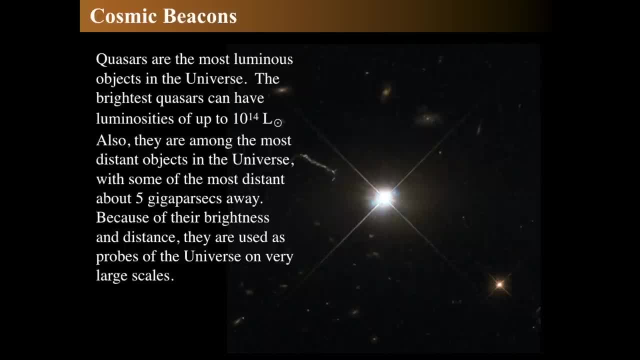 some of them can be up to about five hundred and a hundred and fifty million billion, well, almost 12 billion light, light years away. this is a bit of a large thing to say 15 gigaparsecs, because multiply it by three and you get too far, so I made a mistake with that. it's really a four or five anyway. so 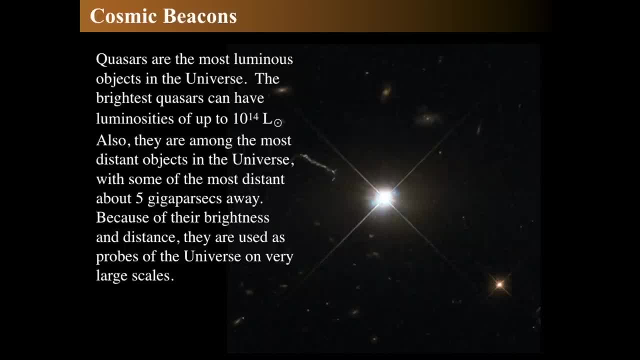 this is 3273. it's still pretty near, but it's luminosity as a point-like object. all comes from the central region, just like we saw in m87 study of the VLA, and that can be a small fraction of this thing, but it can be foldable if we then 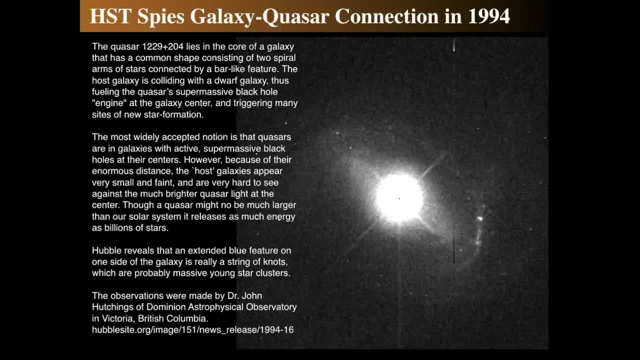 look at other quasars, they actually thought that they were galaxies for a while and couldn't resolve them. so it took a long time for people to actually resolve the surrounding galaxy, because razors are pretty freaking bright, so they're extraordinarily bright objects. and finally, this one was an image that 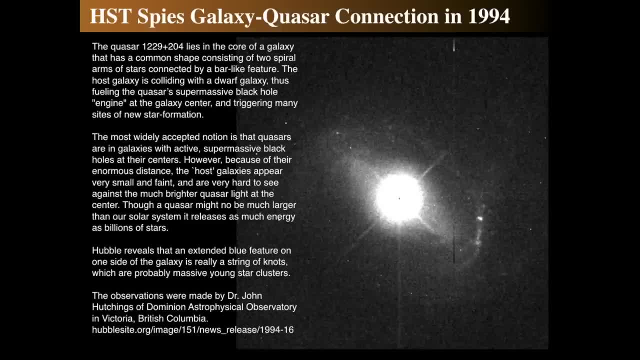 was released in 1994 using the Hubble Space Telescope. there were other. there were other images that showed some pretty good Vas from ground based things that were extraordinarily good studies of these exact things. but then the Hubble spacelishness trading Child's, you know they came to awful. 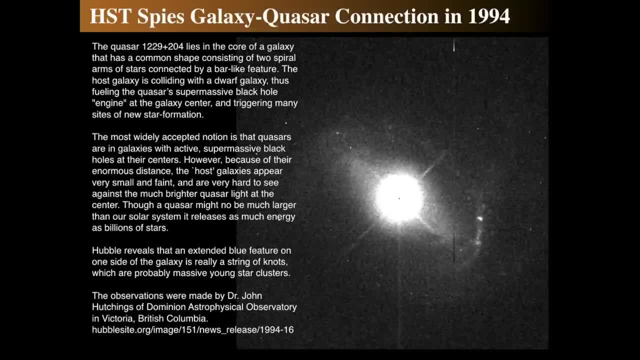 to help establish the their own same together. but sort of same problem can infer here from a rathercross perspective. there does include Clarke vauxville- don't let anyђ sea. telescope confirmed what looks like a bar-like structure in the center of it, all surrounded by what looked like a spiral arms. So we have that there's a. 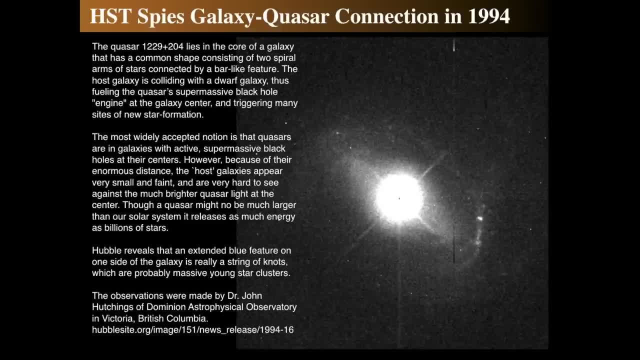 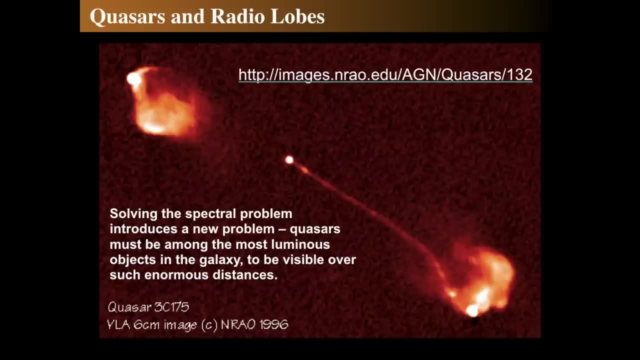 host galaxies with an extraordinarily bright object in the center and this must be a colliding galaxy, and something what's happening is is that the bright the quasar object is the bright central core. Quasars also have radio lobes, and this is another one. this is a quasar, 3C175, taken with the VLA at 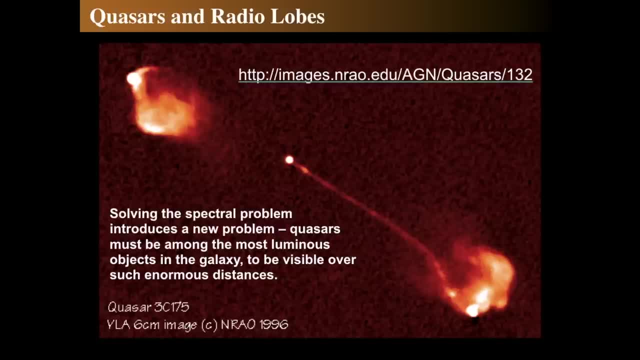 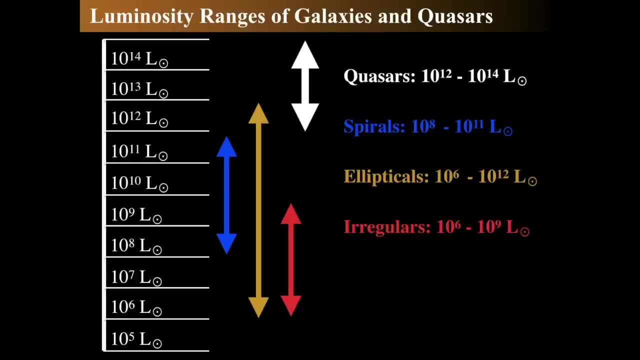 six centimeters 1996, and I provide the link there so you can go hunt it down. and yeah, you can see that quasars themselves, in addition to being bright, bright, bright, luminous sources, are also staggeringly luminous radio sources as well. Alright, so to kind of sum it up, we we discussed in a previous lecture the 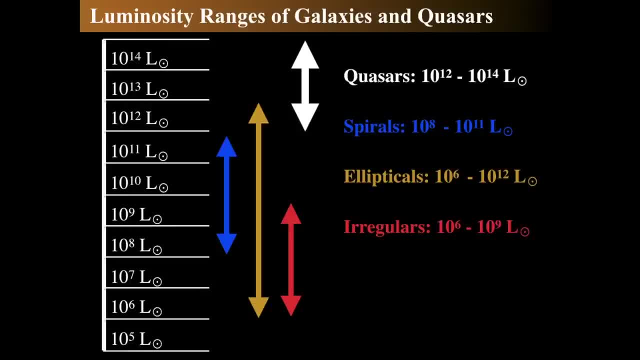 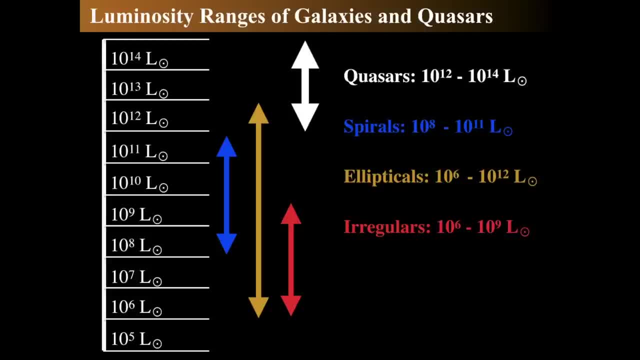 go ahead. the 1,000 Milky Way galaxies are compressed inside an area that we'll find inside a volume that's smaller than the solar system, So this is really catastrophically bizarre that something 1,000 times more luminous than the entire Milky Way seems to be coming from a little volume. 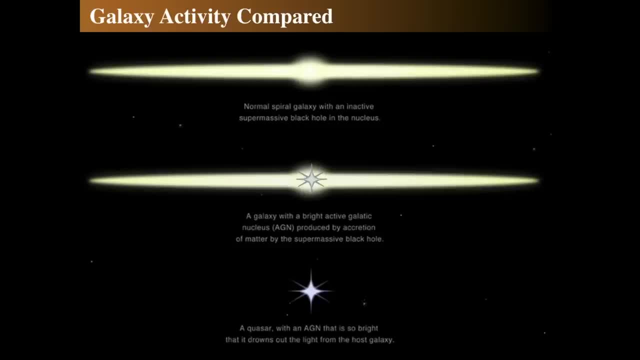 that could fit inside the solar system, All right. so just in rough schematics, normal galaxies just have gas and dust and they've got a nucleus and such forth and you know it's kind of pretty and such forth. But then we look at the edge-on views, of course, If it's got. 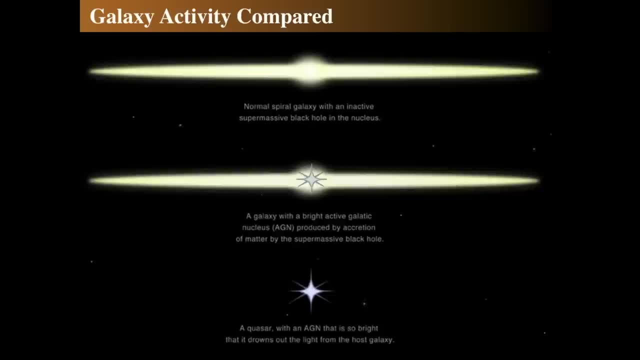 an active galactic nucleus, then the center is really really bright and it's got bright broad emission lines. It's probably formed by something like we call supermassive black hole, which we'll justify next time, But a quasar is so insanely bright it drowns out that thing. It's not that. 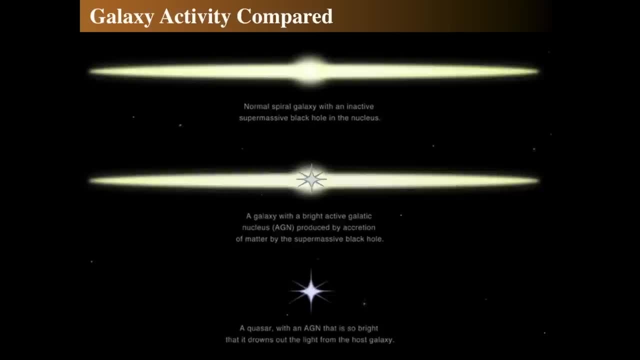 the disk doesn't exist. It's that the contrast is so great that you can't see the disk. It's not that it doesn't exist, It's that it's too bright to see it. So it's like, hey, hey, stare at this light, Stare at my flashlight. Oh, I can't stare at your flashlight.